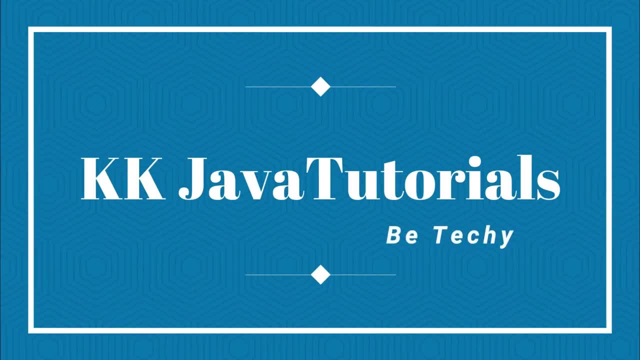 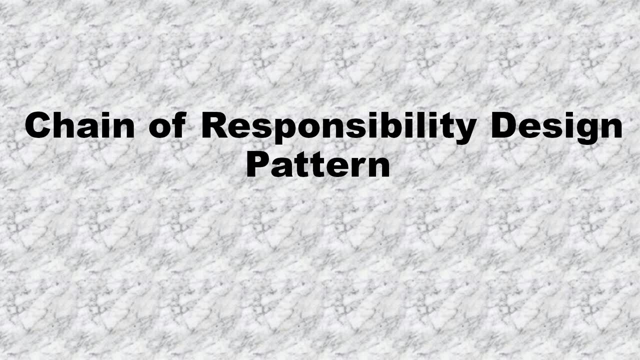 Welcome to KK Java Tutorials. In this video tutorial we will talk about chain of responsibility design pattern in Java. First of all, we will understand what is chain of responsibility design pattern in Java. We will see all the concepts and then we will take a huge guess. 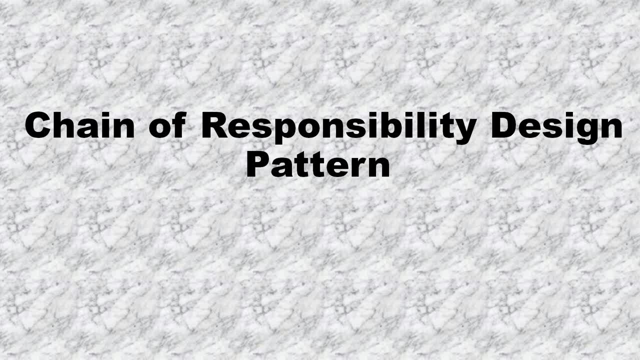 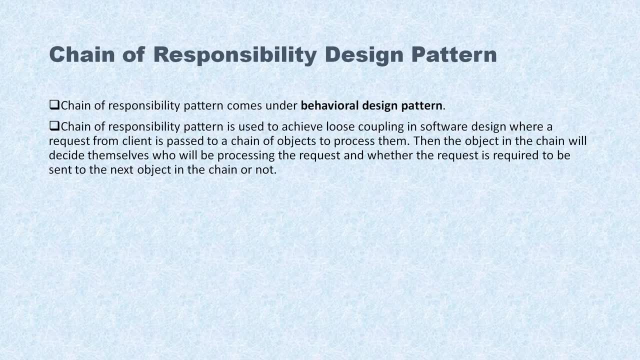 and that huge guess we are going to implement over here. So let's try to understand first of all, what is chain of responsibility design pattern? So first of all you need to keep in mind chain of responsibility design pattern comes under behavioral design pattern. Now 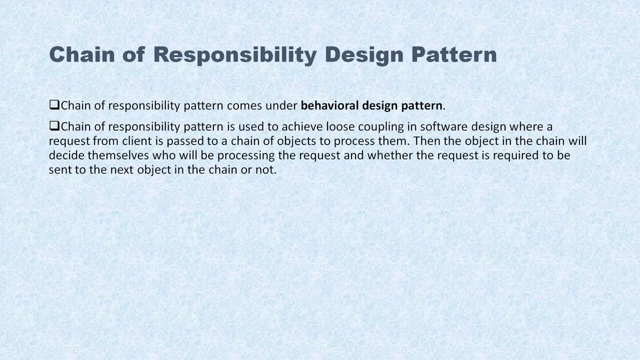 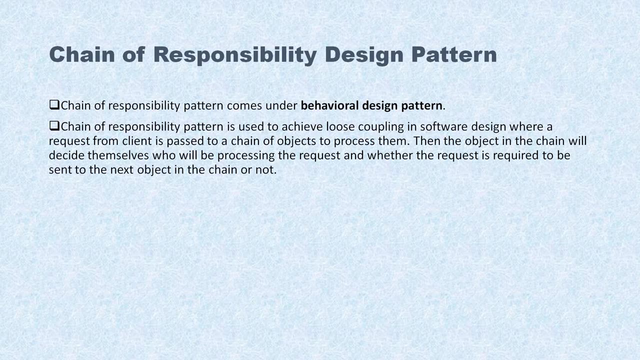 chain of responsibility pattern is used to achieve loose coupling in software design, where a request from client is passed to chain of objects to process them. Then the object in the chain will decide themselves who will be processing the request and then request is required to send to the next object in the chain or not. So this is the concept, all. 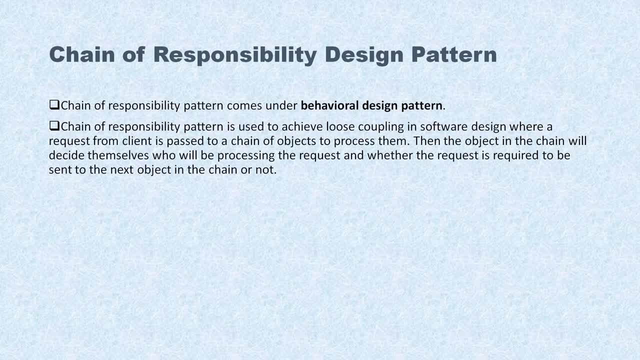 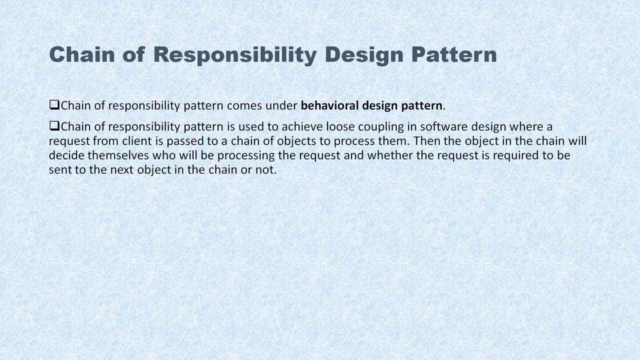 about Chain of responsibility design pattern. One of the beautiful example is filter in servlet, So filter. you have a chain of filters and you pass the request from one filter to another filter and if there is required, then we pass request from one filter to another filter. 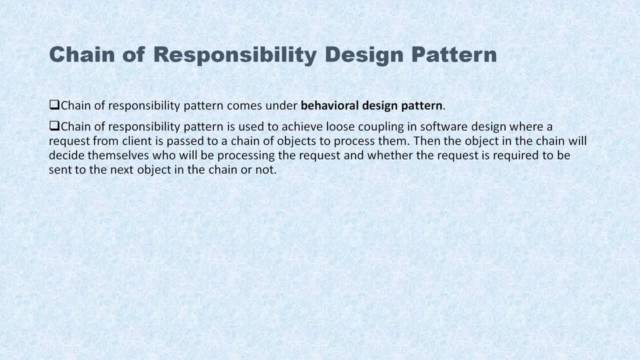 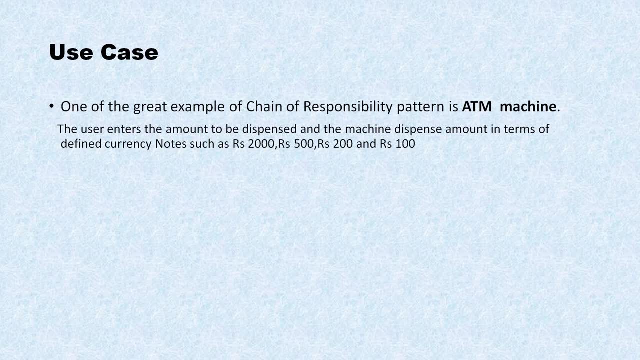 else we can send response back from the first filter itself. So that's the best example of chain of responsibility design pattern. Now, here in our scenario, We are going to implement something is called ATM machine, right? So one of the great example of chain of responsibility pattern is ATM machine. Here user enters the amount to be. 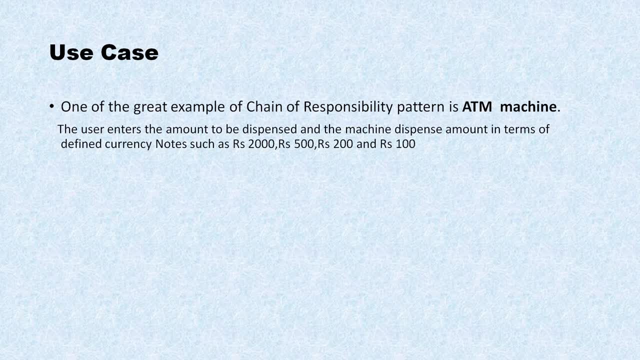 dispensed and the machine dispense amount. in terms of defined currency notes, such as in India, we have four kind of notes in ATM machine: right: Two thousand, five hundred, two hundred and one hundred right. So if you try to enter, if you enter amount, then amount will. 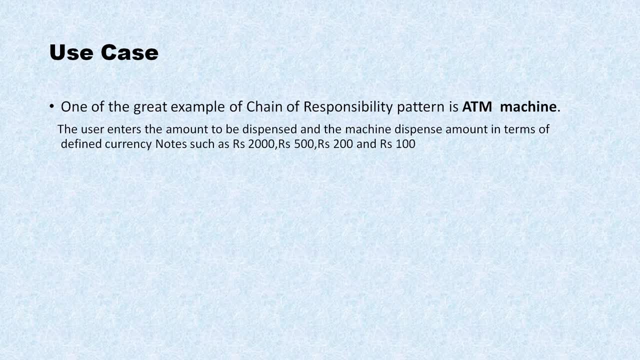 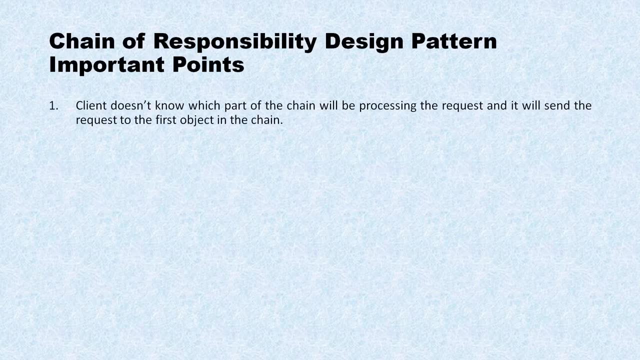 be dispensed in the available currency. Now, before proceeding to implement this design pattern, let's have some some of the important point. First important point: client does not know which part of the chain will be processing the request and it will send the request to the first object in the chain. So client is 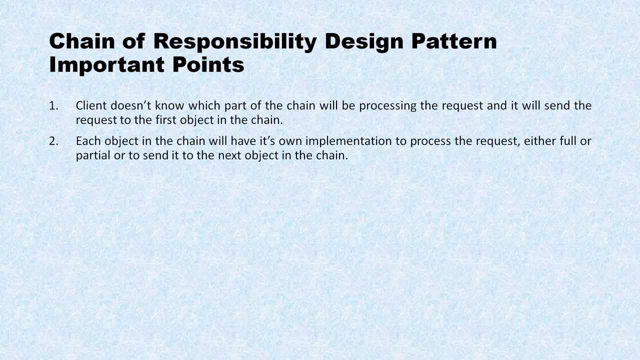 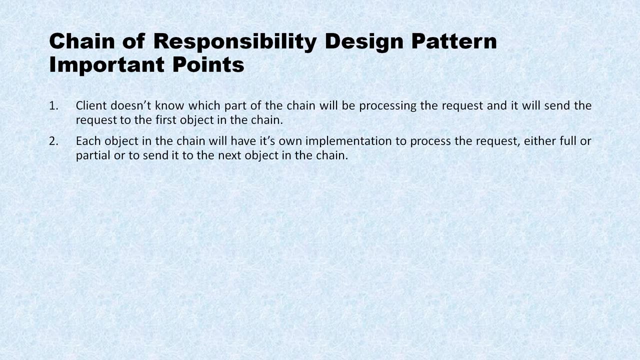 completely unaware about the. I mean which part of in the chain request is getting processed. Each object in the chain will have its own implementation to process the request, either full or partial, Or to send it to the next object in the chain. So here, when you try to withdraw the money, 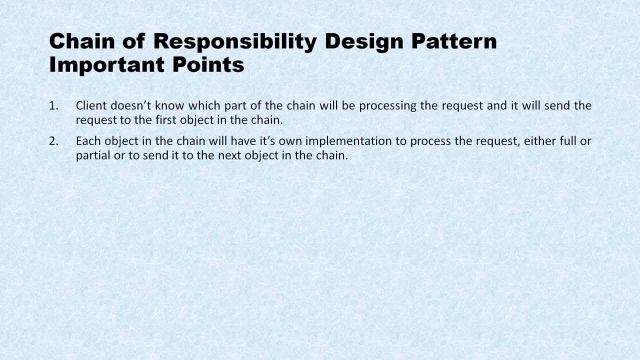 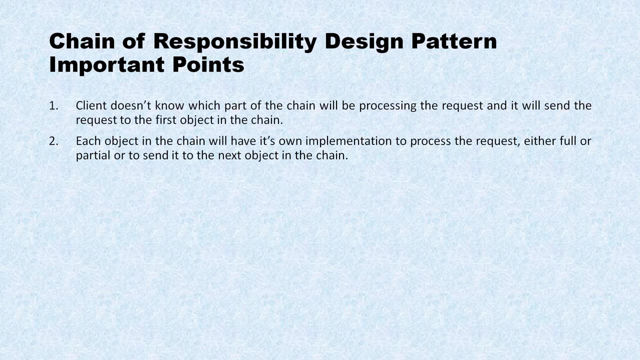 from the ATM right. So if you enter the amount, then that is not. that is not always that request is going to process by the only one processor. There are chain of processor and in sometimes, if let's say, if you are entering 200, then only one processor is able to process your. 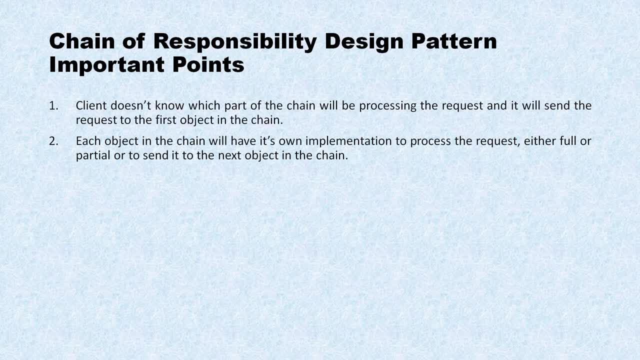 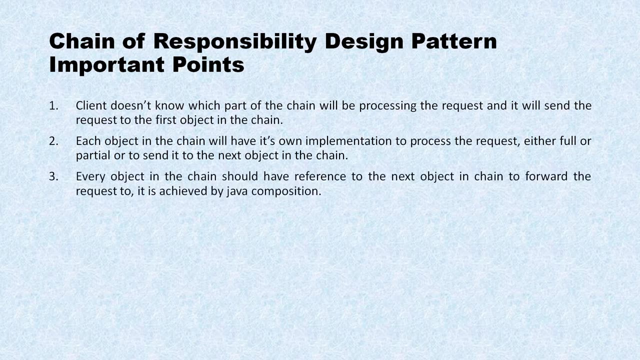 amount. So if you are entering amount like 1500, then there are two. processor comes into the picture Again. that depends on the. what kind of nodes is available in the in ATM right? So that we will see through example Now: every object in the chain should have reference to the next object in the chain. 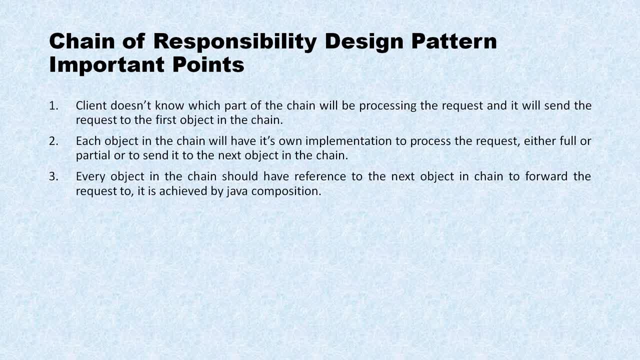 to forward the request. It is achieved by the Java composition, So we will see how we can process the request from one chain to the another chain in the processor. You can do this by using composition. Creating the chain carefully is very important when you. 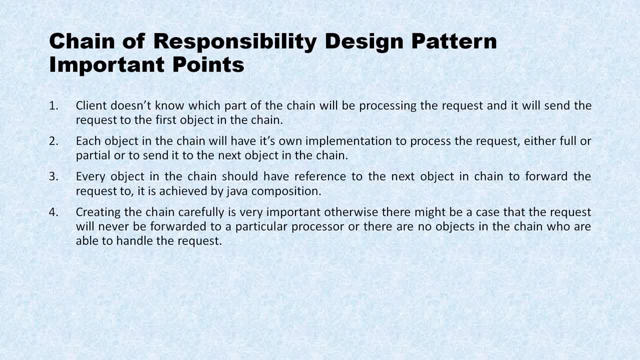 implement chain of responsibility design pattern, otherwise there might be a case that the request will never be forwarded to a particular process. There are no objects in the chain who are able to handle the request right. So let's see these key points. only you will understand. 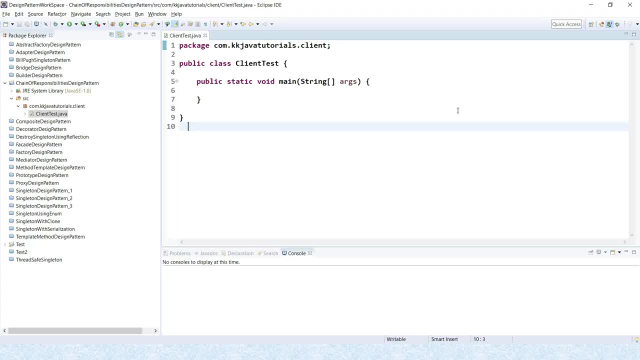 when we will try to implement this design pattern right? So here is the Eclipse, and here I have just created a project with the name chain of responsibility design pattern. Now let's see how we can do it. Here is the Eclipse, and here I have just created a project with the name chain of responsibility. 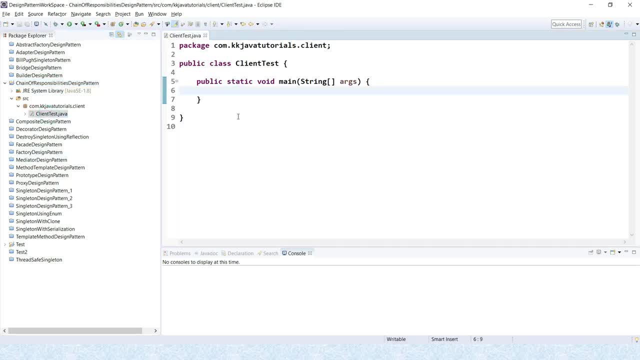 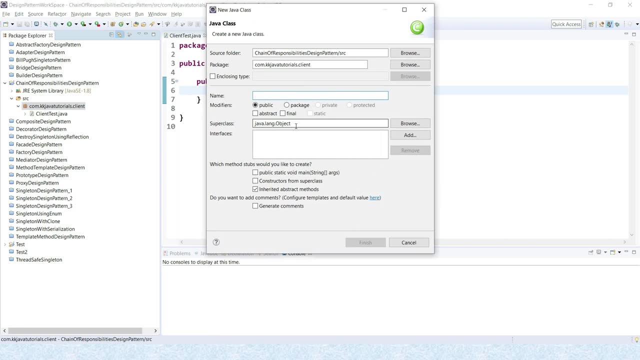 design pattern. So let's see how we can do it. So let's see how we can do it. So let's, And here just I have created a client program, nothing else. Now we are going to implement each and everything from scratch. So, first of all, what we have talked, we are going to implement ATM machine over here, right, And ATM machine will have a four kind of nodes: 2500, 200 and 100.. What nodes are available in the ATM in India, right? 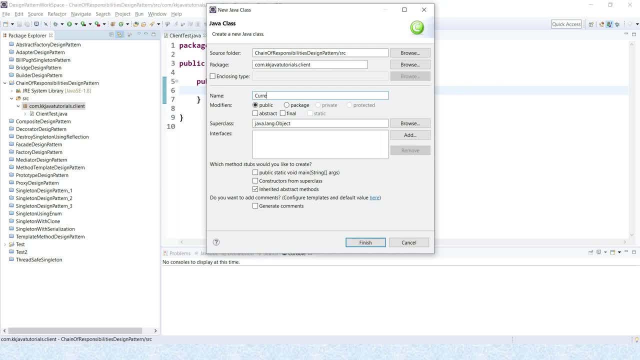 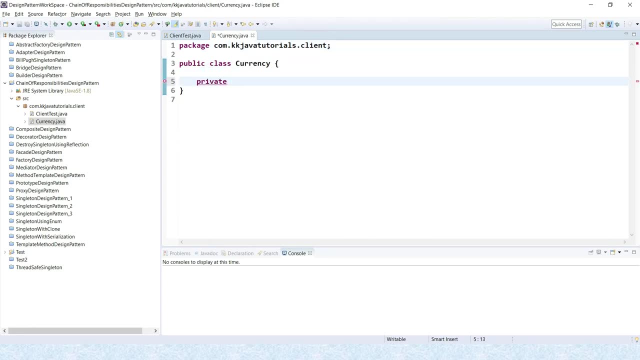 So first of all I'm going to define a class. it's called currency, Okay, And this class will have one variable, is called amount. Anything you can give here amount would be. giving a name as amount would be meaningful, And here I'm going to create a constructor to initialize this amount. Yeah, And now let's say we have a getter method: get amount as well. 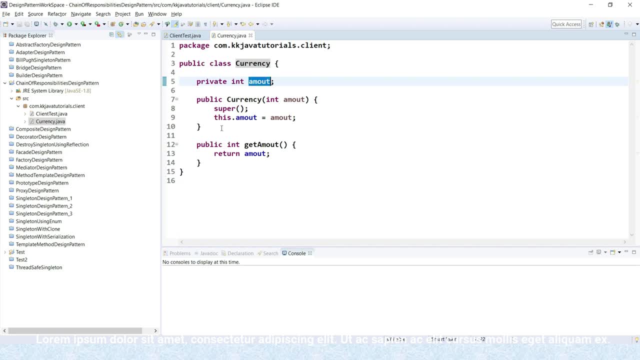 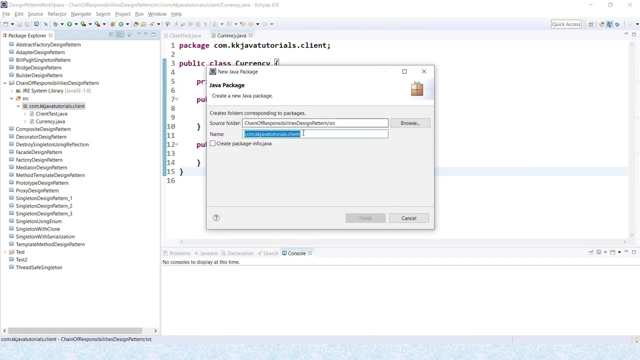 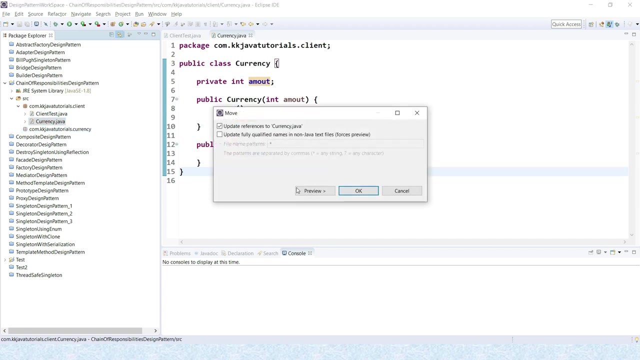 Cool, So simple, Simple class currency which will have amount, public constructor and getter method. That's it. This amount is going to use by a chain, right? So here now what I'll do? I'll create a separate package, I would say currency, And there I'll dump this class. Okay, Now I'm going to create a, basically a currency. 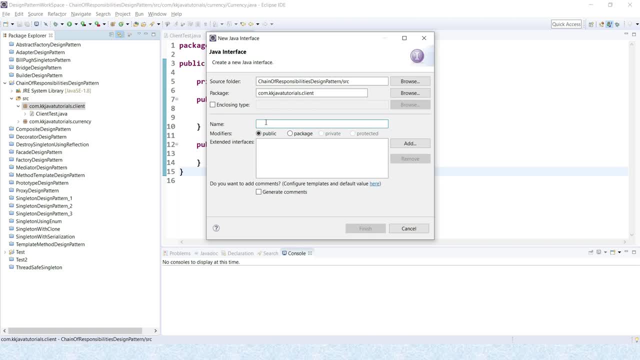 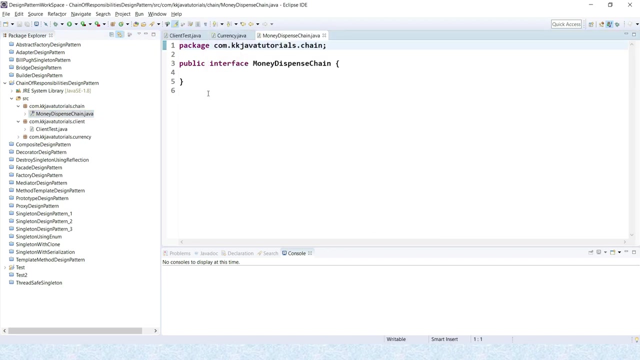 And here I'll give and package, I'll give chain, And here I'm going to give that interface. now, name is called money dispense chain, because this chain is going to process money, right, Money dispense chain. Okay, and here this guy is going to declare two methods: public struct void. first, 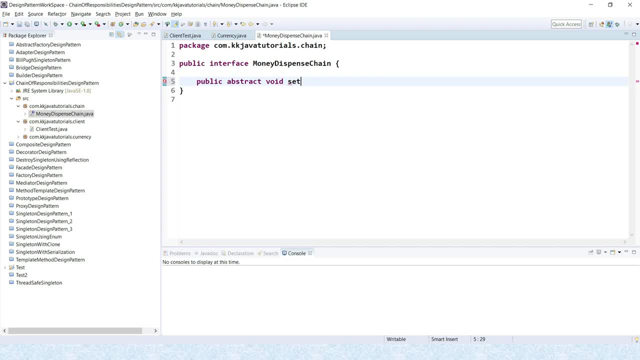 method we are going to define set next chain right, and this will have a reference of money dispensing. okay, and next method we are going to define. method is called dispense- dispense- which will have a reference of currency. cool, so there are two method. now we'll have a. we have to define a different color. 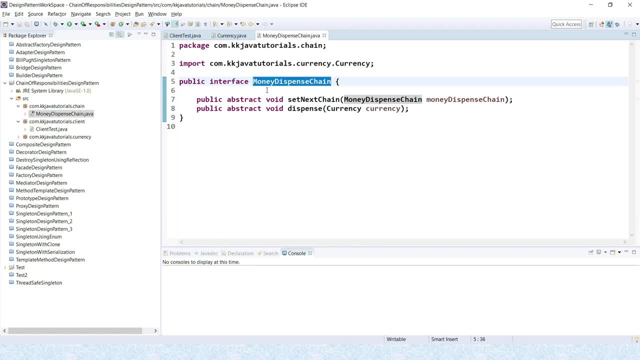 right which is going to implement this money dispensing and as we know that in India we have a four kind of notes in ATM machine: 2000, then 500, 200 and 100. so we are going going to define for processor, in this case, so to process a 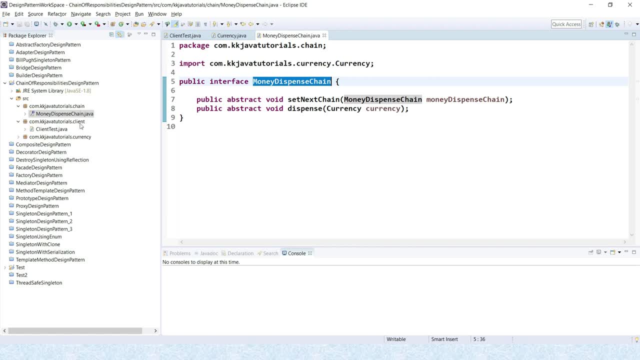 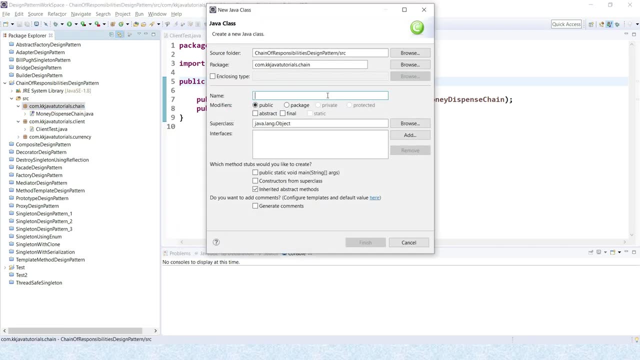 2000 note. we required a processor which will process 2000 note. right, so I'm going to create a class and this IMPL package, and I would say it's not meaningful. but but here, money, what I'd say, not money, I would say rupees. let's say the rupees two thousand. 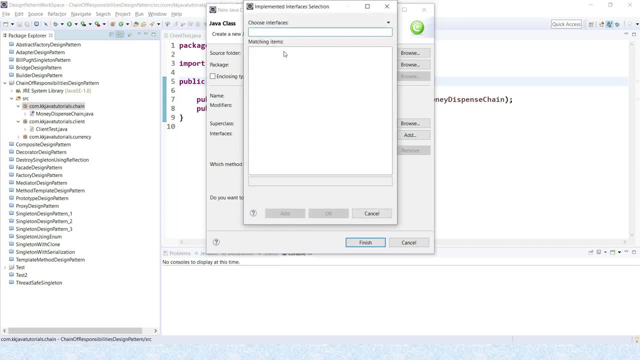 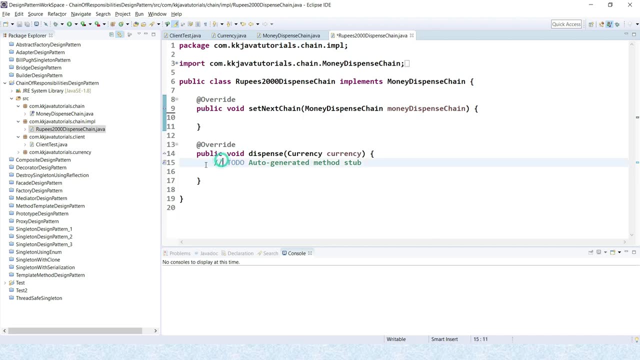 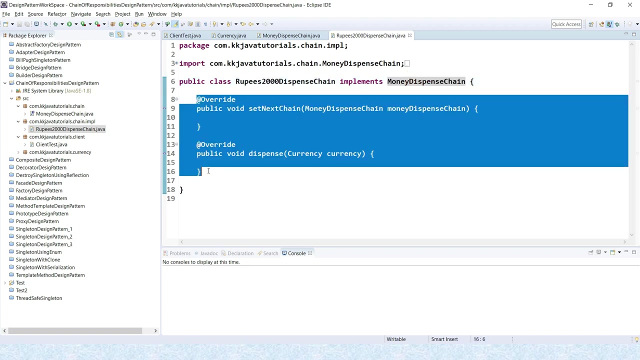 dispense chain. right, that's looks like meaningful. now this guy is going to implement this interface: money dispense chain- right now. here, if it. you can see now as we are implementing this interface, right. so this interface is having two methods. these methods we have to define, right, so here I'm going to. 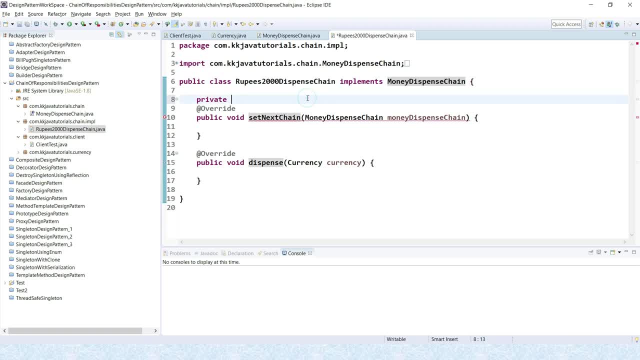 declare private and this money dispense, sorry, that's okay. now here in this method, what I'm going to? this dot money dispense chain equal to money dispension, cool, now in dispense method also, we have to provide the some business logic, right, that's very important. so here I am going. 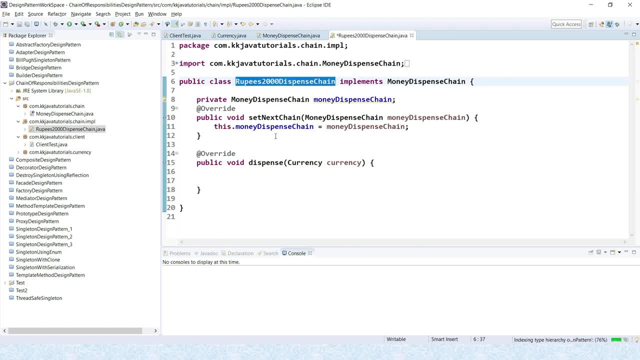 to first of all check, as we have created this class to process 2,000 notes, right. So here I am going to first. if in this currency I am going to look what's the amount is coming, get amount is greater than equal to 2000, then I am going to write some business logic inside. 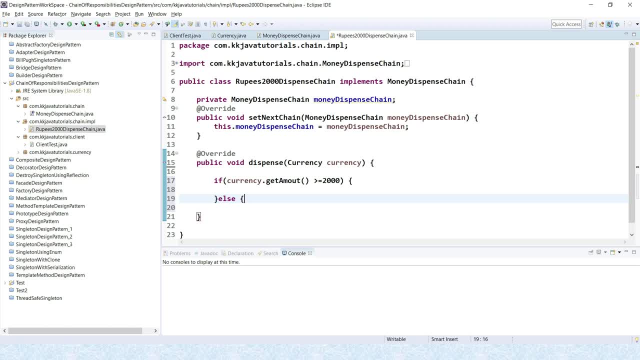 that else, if processing amount is less than 2000, then we need to send, we need to basically forward request to the next processor in the chain. right, so that how we can do that, that we can. we have a reference of money dispense chain dot. I would say dispense and of course, 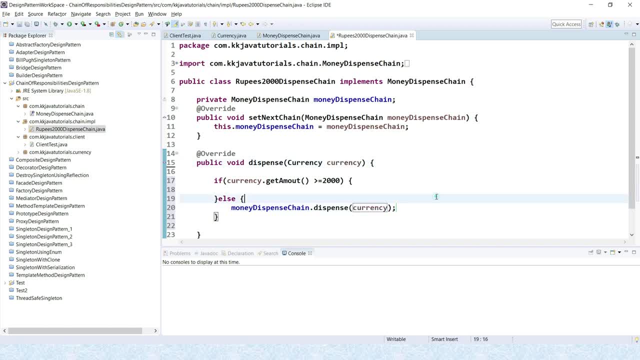 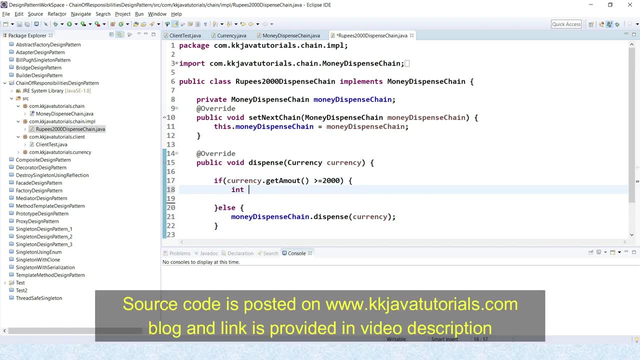 we need to pass this reference of this currency equal straight forward now here. if amount is less than 2000, then what we are going to do, first of all, int, I would say number of notes Equal to currency, currency dot. get amount divided by 2000 right. in that way we can get: 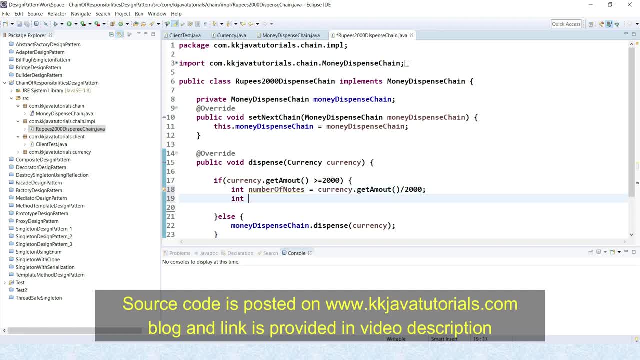 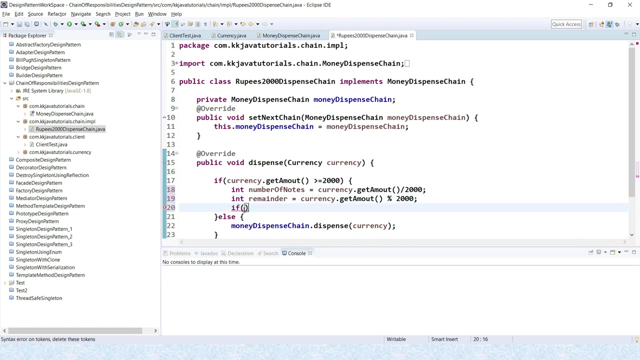 the number of notes and afterwards what we have to do. remainder, we can also check remainder. remainder equals to, again, currency, dot, get, amount, and here we will do modulus division right, modulus division of 2000, which will give us the what's the remainder right, right. so here again we will check: if this remainder, this remainder, not equal to zero, then what? 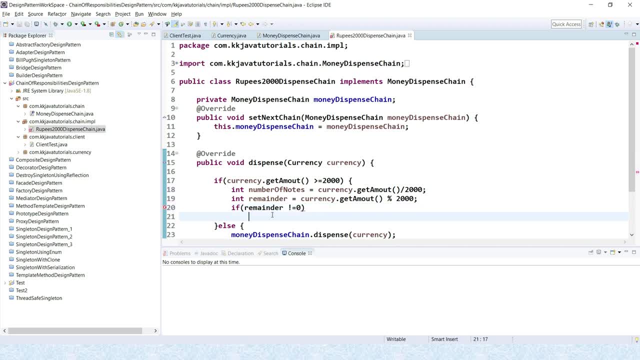 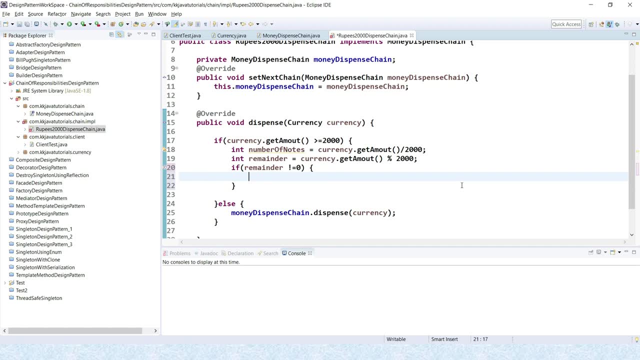 we have to do? if remainder is not zero, then we have to forward the request to the, basically the next processor. So here again, we will check if this remainder, this remainder not equal to zero, then what we have to do Now. here again, it should be fun to the this divisor chain, I would say here: 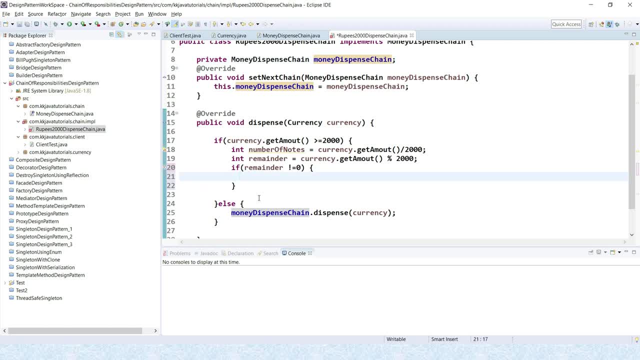 Let say: dispense the chain right, this is dispense. Say this even: potential of the chain exchange in not equal to zero and what I would say dispense師 and defendors we have to deal with up to here and another state accounts machines. 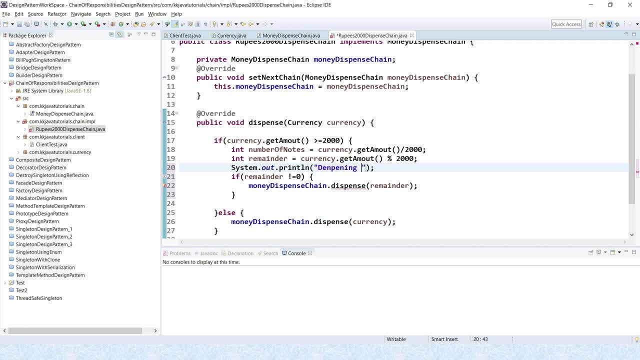 dispensing, dispensing. give some space so that number of nodes of rupees 2000,. write. this will print. if you enter amount is 2500, right. so here this guy is going to print: dispense, sorry. dispensing. dispensing to right. dispensing to nodes of rupees 2000,, right. 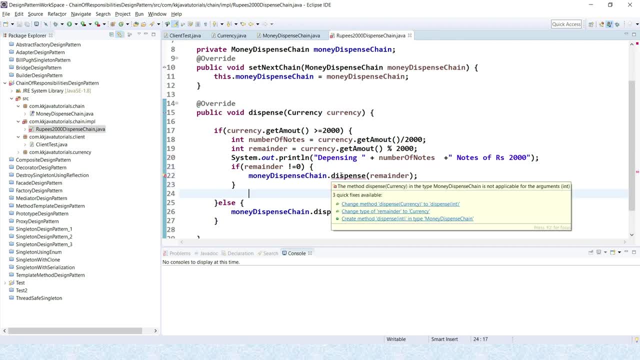 and here if remainder, if remainder is not zero, then in this chain we are calling dispense method. but here we have to pass the new currency amount, new currency object, and here we will pass this remainder. right now we will create. 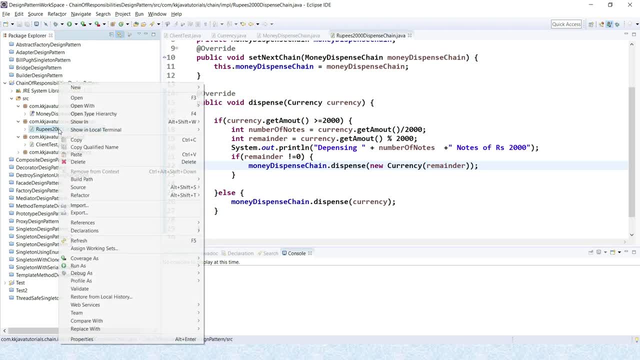 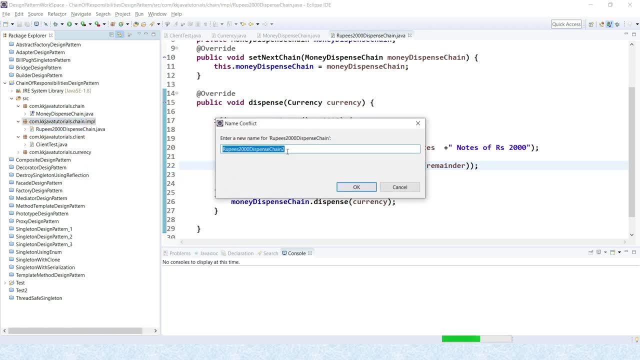 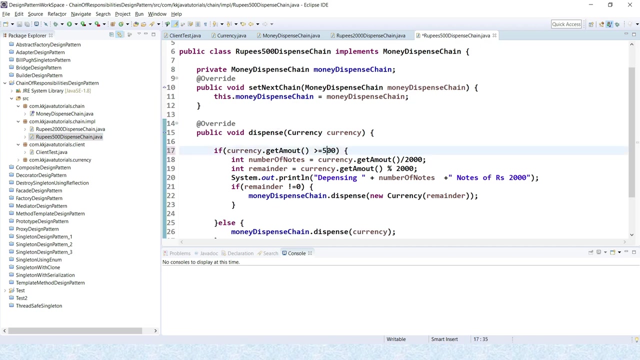 few more classes. so this is going to process node for 2000,. again, I am going to paste this guy- I will give the name- which is going to process 500 nodes: 500 nodes. so another class here. few changes we have to do. amount is greater than 5000, then 5000, wherever. 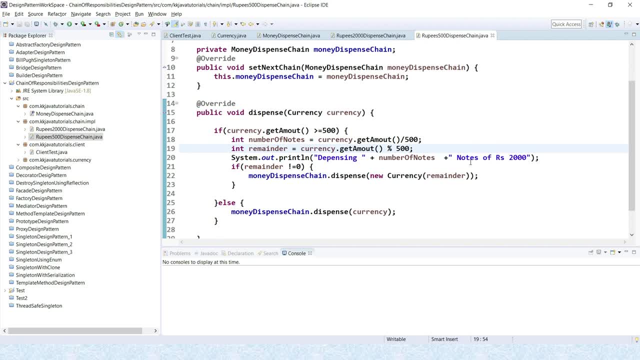 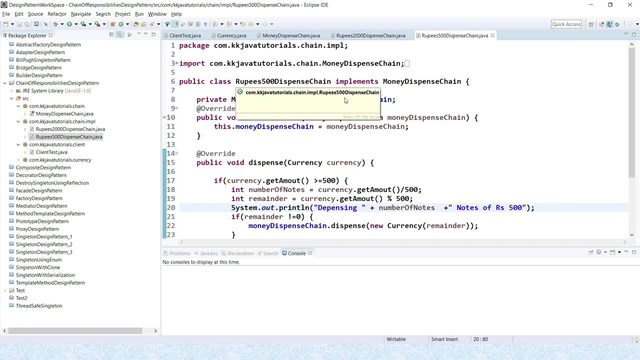 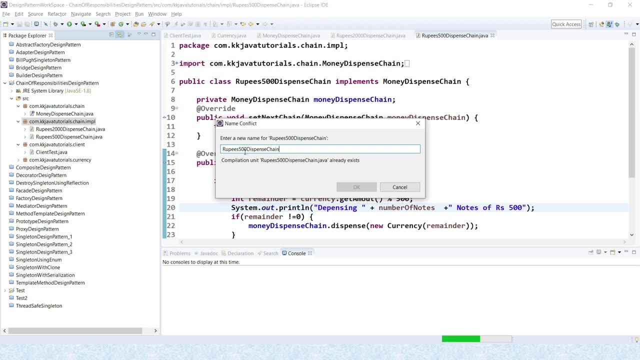 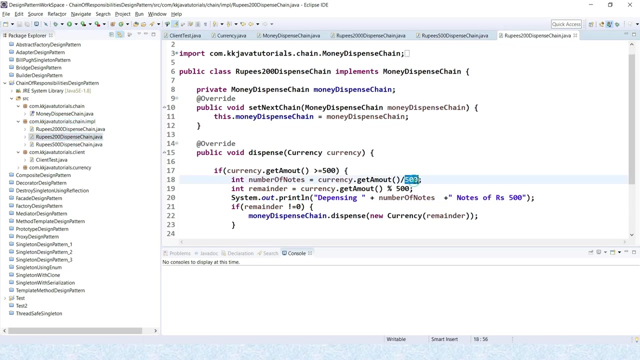 2000,. 2000, replaced with 500,- sorry, 500, nodes of 500,. so this is basically class which processes 500 nodes. now again we have to create another class which will basically process 200 nodes. right, so, 200 nodes, and for 200, here we have to specify 200, where. 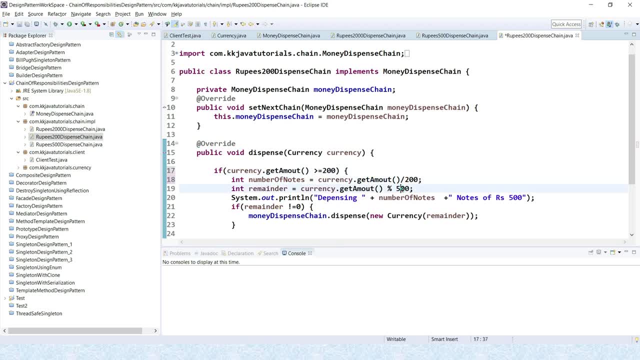 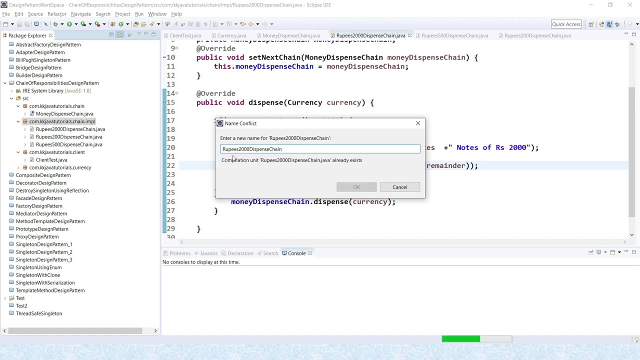 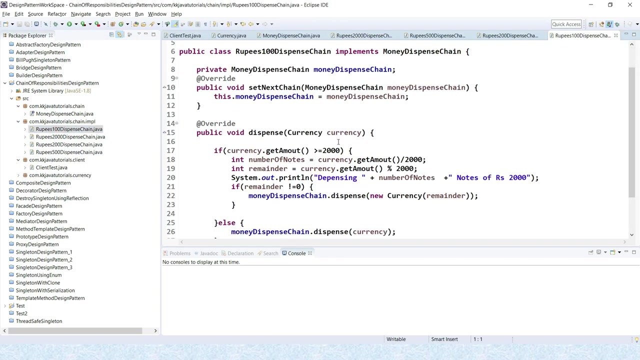 500 replaced with 200, that is cool. And now we are going to put 200 nodes. So this is it, that's it. and finally, we have to create one more class which will process hundred rupees, note right. so I would say hundred rupees or rupees hundred is mentioned, and here this: 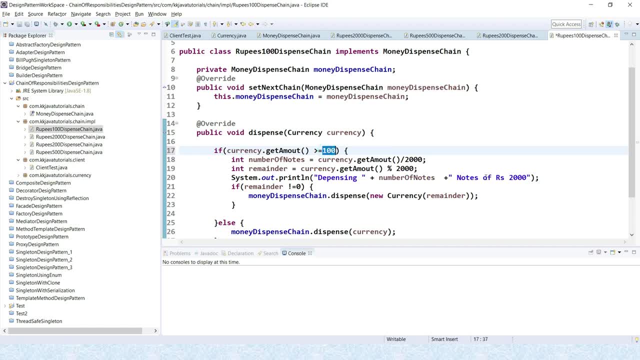 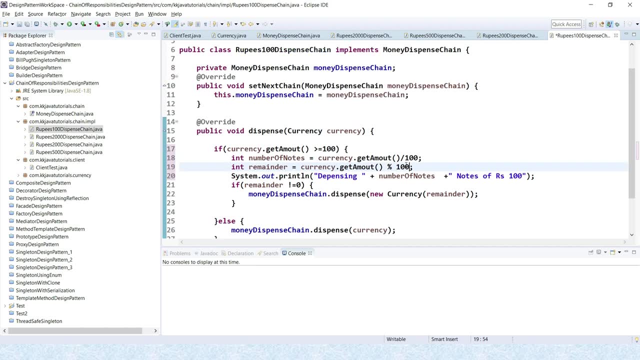 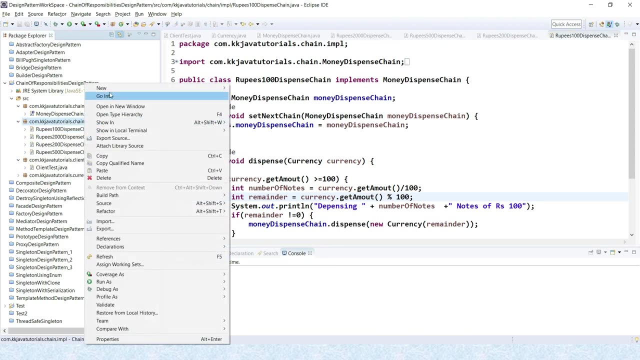 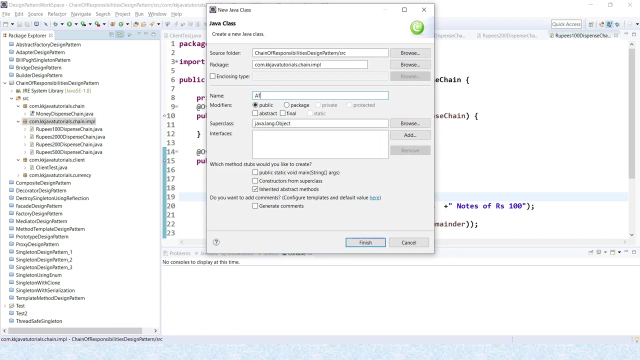 should be hundred. we place two thousand hundred everywhere and we have almost done so. we have created four processor class for four type of nodes. right now I am going to create one more. class is called something. something is called ATM machine. you can say: ATM machine dispense. 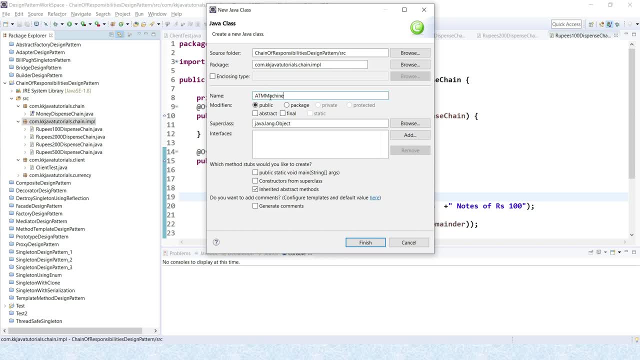 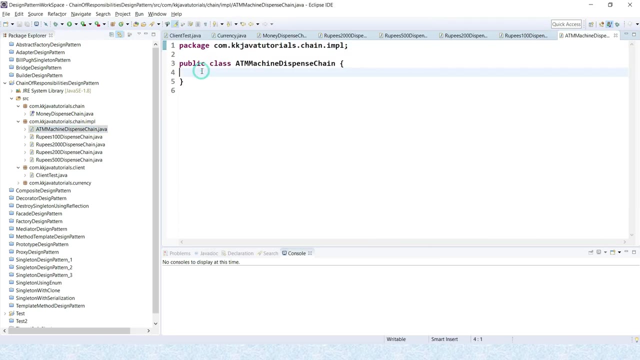 you can say ATM machine dispense and then here I am going to enter my ATM machine and can give. here I'm going to specify ATM machine, that's it. or meaningful name would be ATM machine dispense dispense chain. that would be the meaningful name. okay, now here I'm going to declare private and will create a reference of. 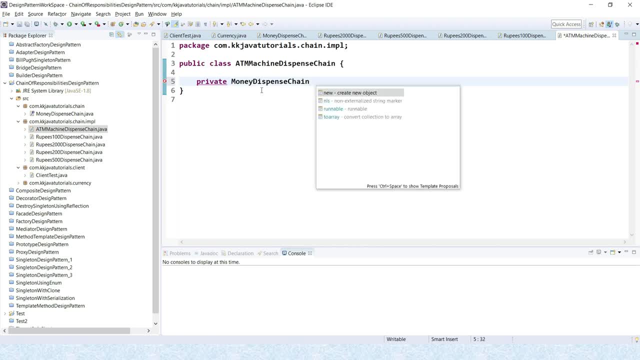 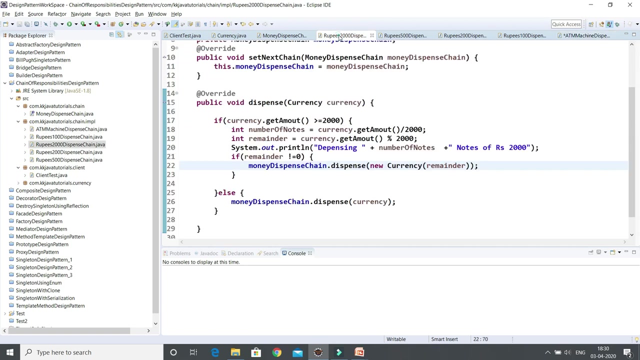 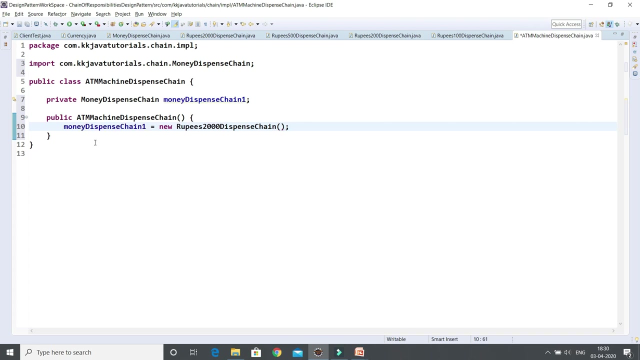 this guy and this would be the chain one. yeah, now I'm going to create a constructor of this guy, this class itself, and here this first chain. I'm going to initialize with new two thousand nodes. this is the implementation for processing two thousand nodes, right? so I would say new 2000. yeah, now I need to create four chain, right. 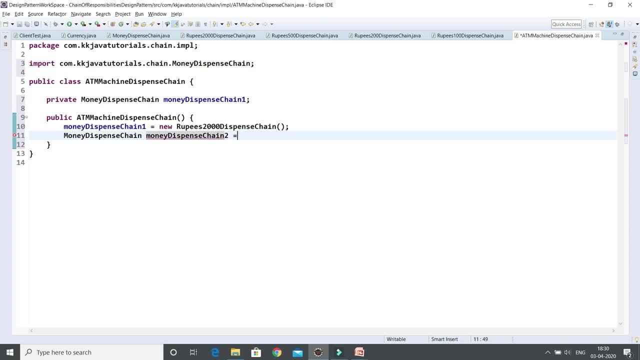 for all four nodes. so I'd say this is chain 2 and I will initialize with rupees. so rupees 5, that next chain I'm going to for 200 right. so it's a chain 3 equal to new rupees process for 500 and 5. so sorry, after 500 we have a 200 right process. 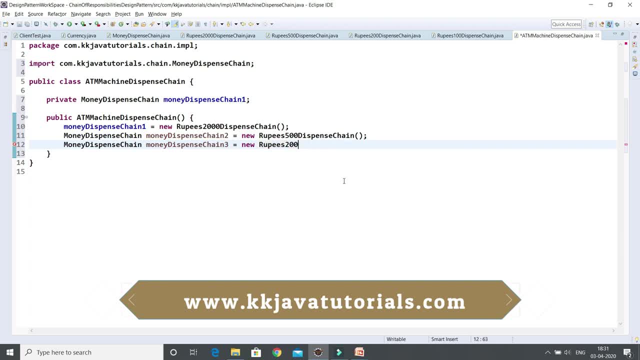 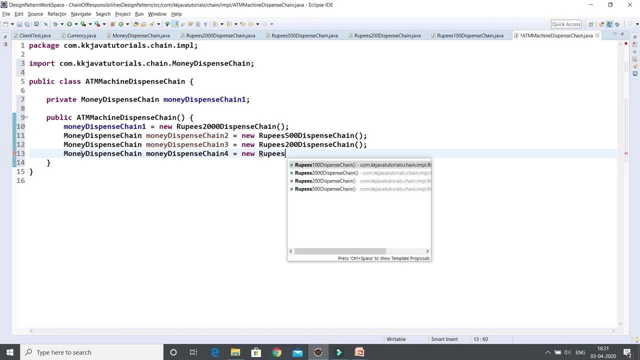 over 200. 200, it's not 2,000, sorry guys. so first processor we have assigned with 2,000, then 5,000, that 200 and finally, third chain would be third. no, third, fourth chain would be new for 100 rupees notes. right, so now what we have to do. 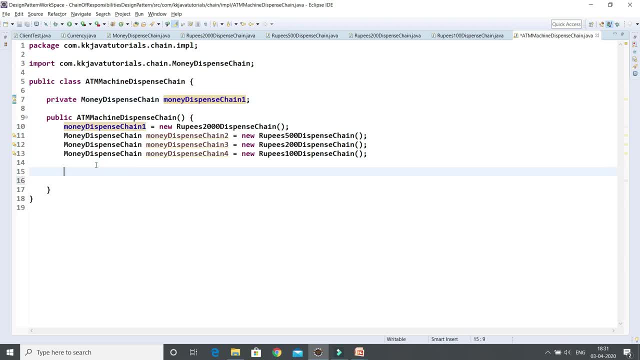 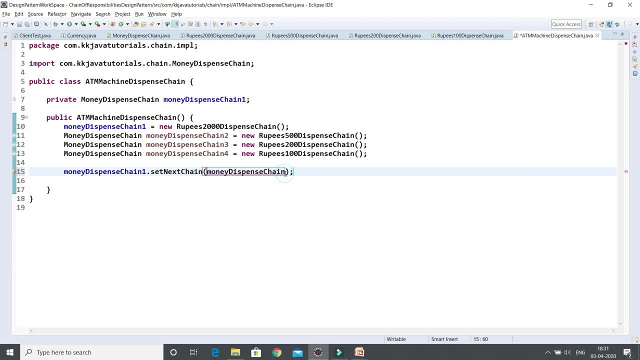 will call the display and sorry a set. will call the display and sorry a set. chain method. right shapes chain and chain method. right shapes chain and chain method. right shapes chain and second shade a chain would be how to second shade a chain. would be how to second shade a chain would be how to change to right and similarly. just I'm. 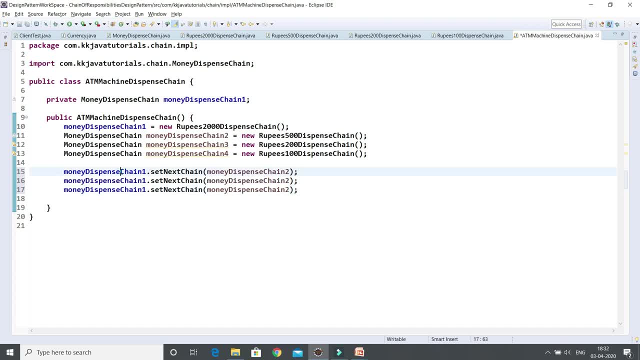 change to right and similarly, just I'm change to right and similarly, just I'm going to copy paste over here this line, going to copy paste over here, this line, going to copy paste over here, this line. so first chain is sending request to the. so first chain is sending request to the. 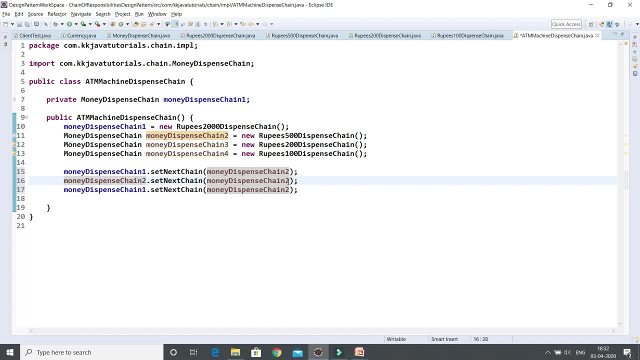 so first chain is sending request to the second chain, then second chain would send second chain, then second chain would send second chain, then second chain would send request to the third chain and third request to the third chain and third request to the third chain and third chain will send request to the fourth. 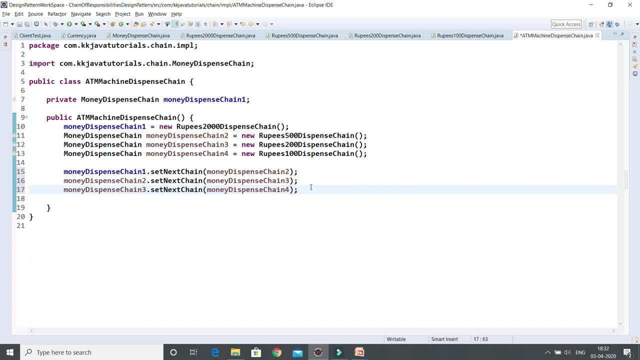 chain. will send request to the fourth chain. will send request to the fourth chain. right cool, this is very simple. chain, right cool, this is very simple. chain, right cool, this is very simple. right now we'll have a client program. so right now we'll have a client program. so 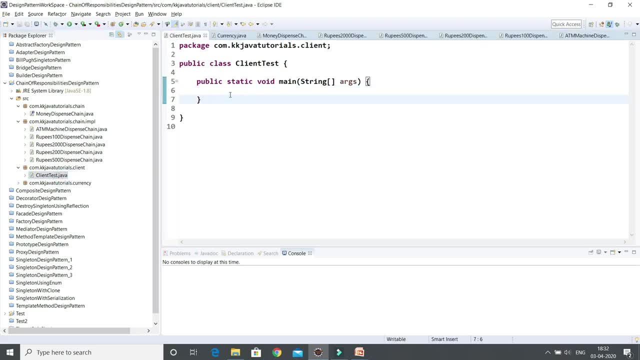 right now we'll have a client program, so I'm going to use client for client, I'm going to use client for client. I'm going to use client for client program over here in this client program program over here in this client program program over here in this client program. what we'll have to use, you can use ATM. 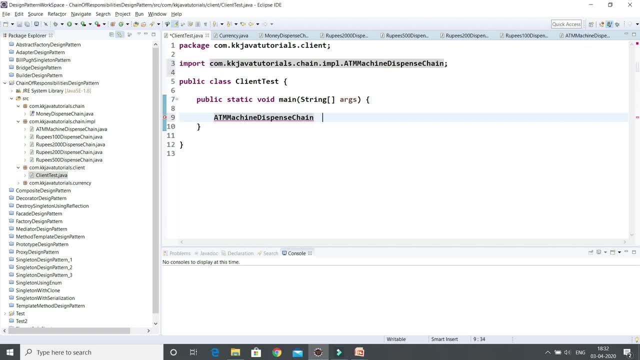 what we'll have to use. you can use ATM. what we'll have to use, you can use ATM, ATM, ATM, ATM machine dispense chain. equal to new ATM machine dispense chain, equal to new ATM machine dispense chain, equal to new ATM machine dispension. yeah, now here what we. 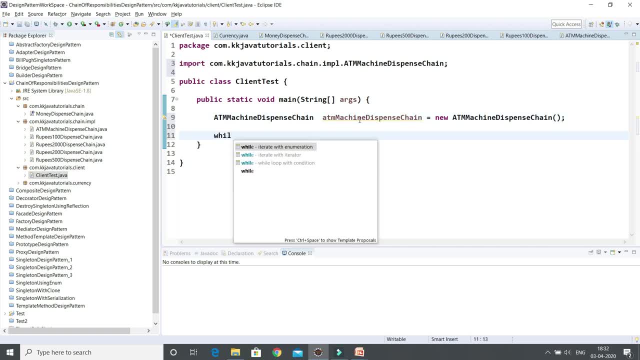 machine dispension. yeah, now here what we machine dispension. yeah, now here what we can do. we can have a one loop while loop can do. we can have a one loop while loop can do. we can have a one loop while loop. this is I'm going to follow forever, true. 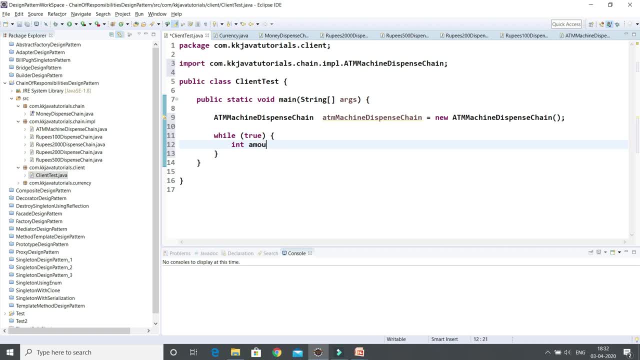 this is I'm going to follow forever. true, this is I'm going to follow forever. true, and here in amount. and what is a sign. and here in amount. and what is a sign. and here in amount. and what is a sign inside with zero. here we are going to. 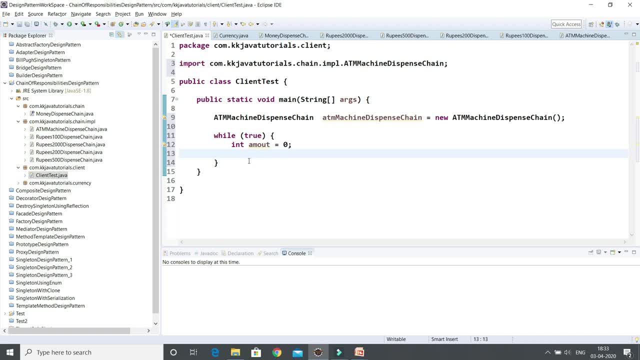 inside with zero. here we are going to inside with zero, here we are going to make use of, let's say, we can make use of. make use of, let's say we can make use of. make use of- let's say we can make use of- scanner. right, 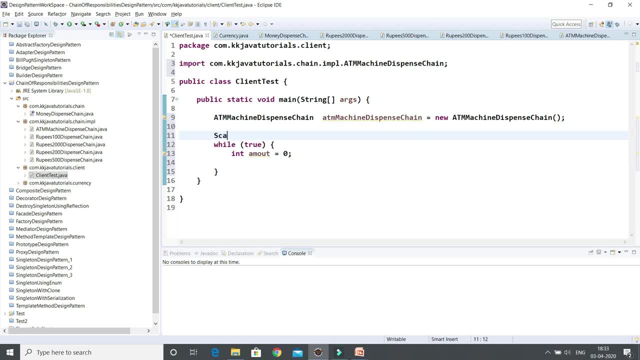 scanner right, scanner right. so a scanner I'm going to miss lies over, so a scanner I'm going to miss lies over, so a scanner I'm going to miss, lies over here. scanner scanner equal to no good here. scanner scanner- equal to no good here. scanner scanner equal to no good. now a scanner we can use over here: new. 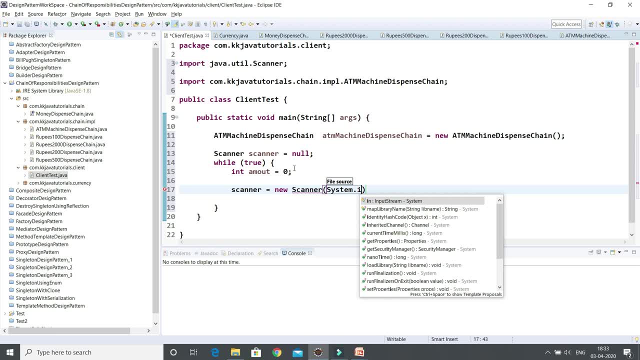 now a scanner we can use over here. new now a scanner we can use over here. new, scan system dot in. because we want to scan system dot in, because we want to scan system dot in, because we want to take input from the system. good, now what? take input from the system. good, now what? 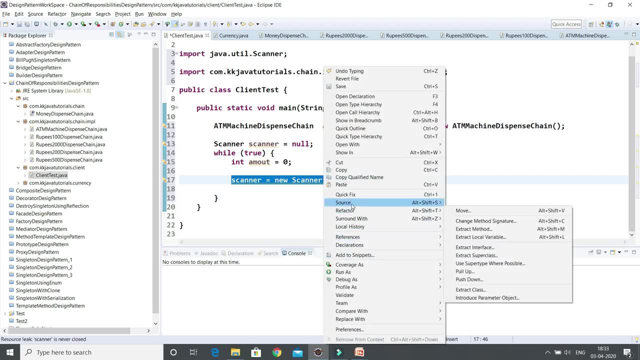 take input from the system. good, now what we can do. we can wrap this guy inside a. we can do. we can wrap this guy inside a. we can do. we can wrap this guy inside a. try catch, try catch, try catch. surround with try catch. yeah, so in. finally, 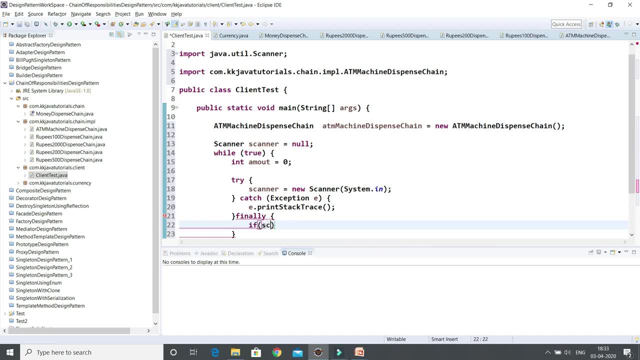 surround with try catch. yeah, so in finally surround with try catch. yeah, so in finally block what we can do if scanner block what we can do if scanner block what we can do. if scanner not equal to, not equal to null, then we not equal to, not equal to null, then we. 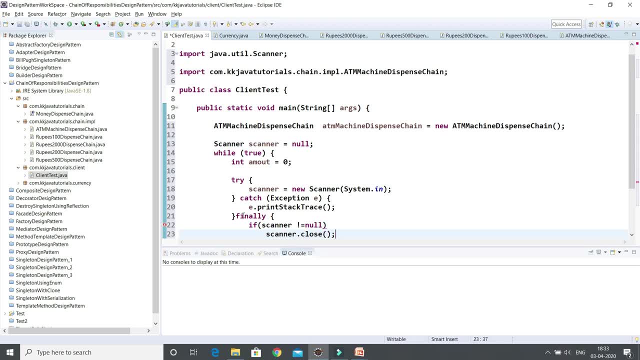 not equal to not equal to null, then we can close this guy. okay, now here we can close this guy. okay, now, here we can close this guy. okay, now here we have a before system dot in what we have, have a before system dot in what we have. 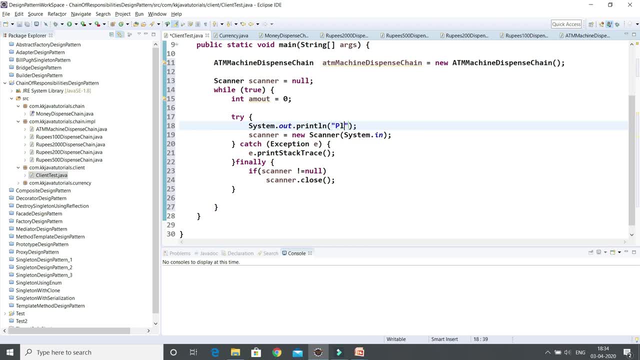 have a before system dot in what we have to print a message. to print a message, please enter amount to dispense. or you can write enter with double amount as well. right now, here we are making use of a scanner to get input from the keyboard, so next int and we get the amount here. right now we have amount now. 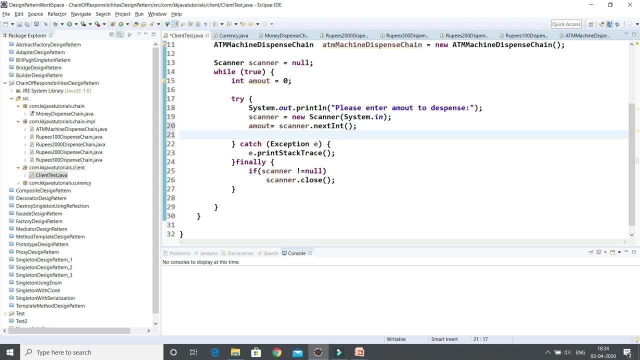 what we have to do basically here we have to check. so if amount should be always multiple of hundred, if that is not the case, then we have to terminate the process. so this amount we have to check. if this model is correct, then we have to check. if this model is correct, then we have to check. 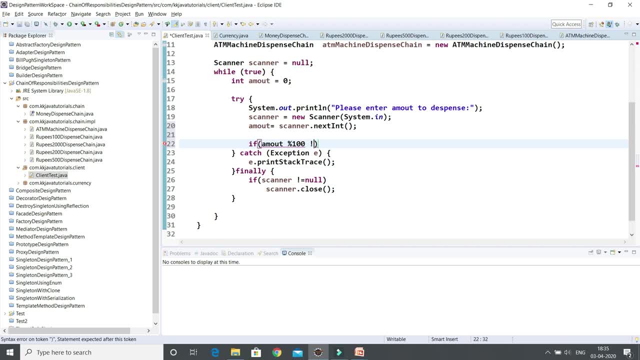 division of under not equal to zero, and that's what ATM works. ie semua. so here, simply, we can prompt the message. here simply we can prompt a message: amount should be multiple of rupees, amount should be multiple of rupees and get the additional amount inside 500. 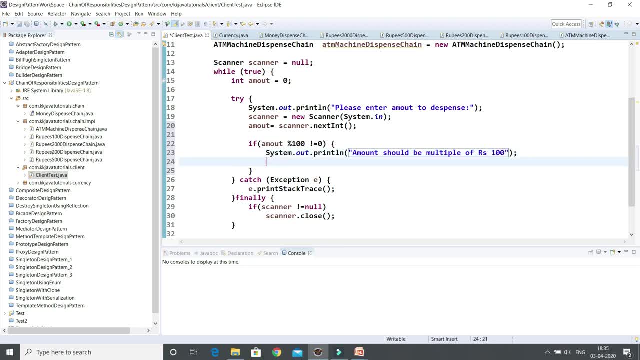 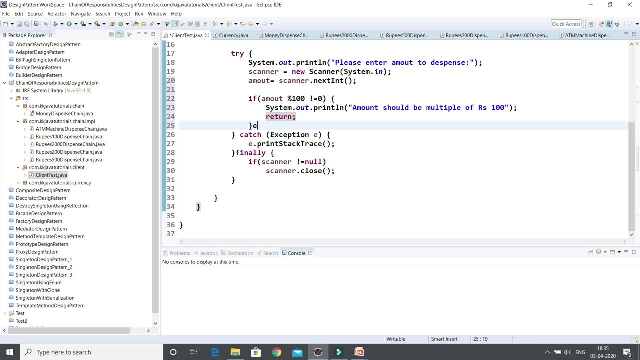 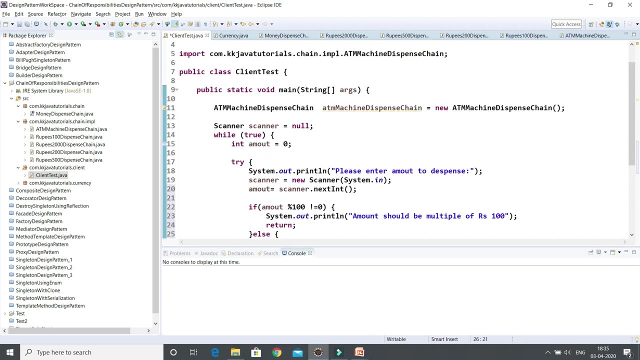 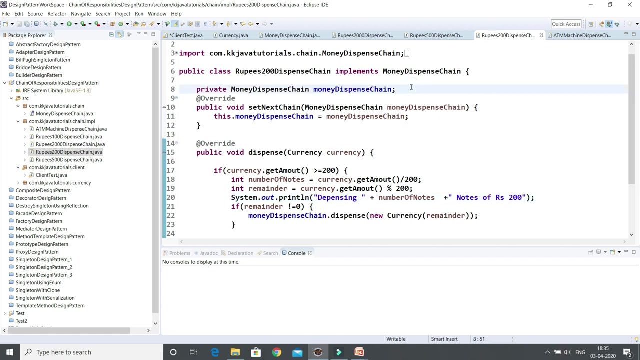 100 right, and if that is not the case, then we can simply turn in the process, else What we will do, Else What we can do. so here, here, The Here, We have this reference right. this reference is a private we cannot access, so we can have a gator method of this guy. 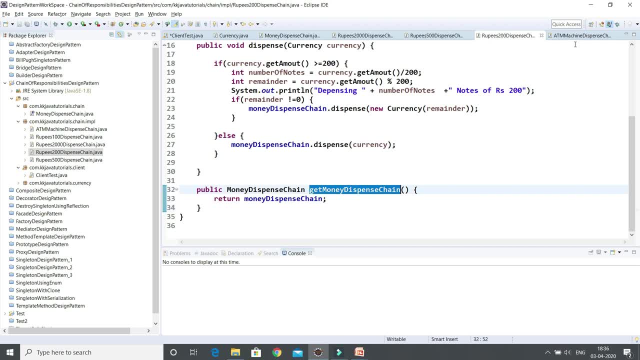 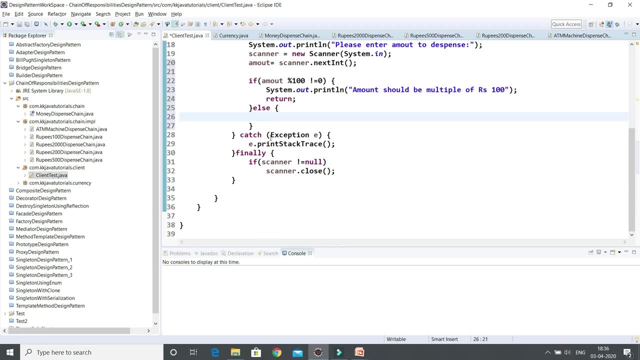 Cool, now what we can do. we have a gator method of this money defense chain. So this Incline program, Let's go to the client program here in else part What we can do. We have a reference of this. You can call its gator method. 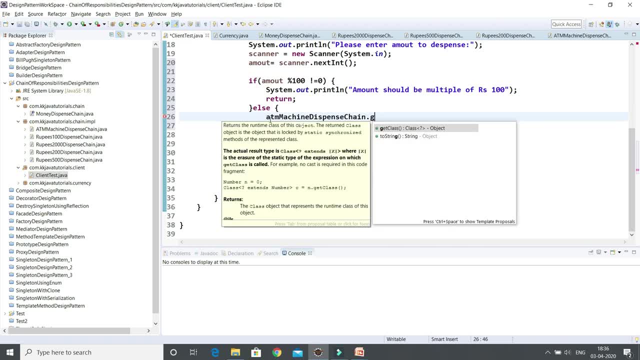 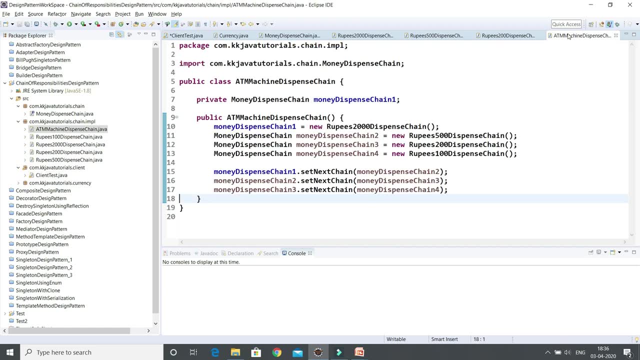 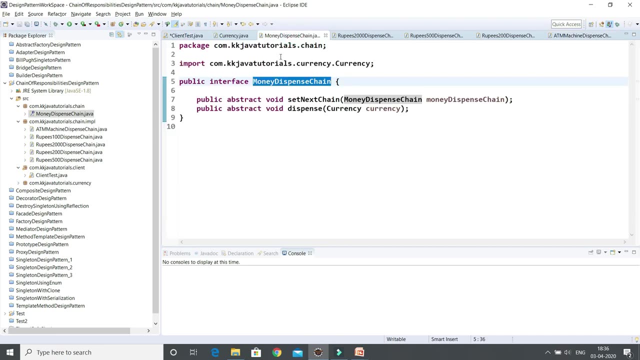 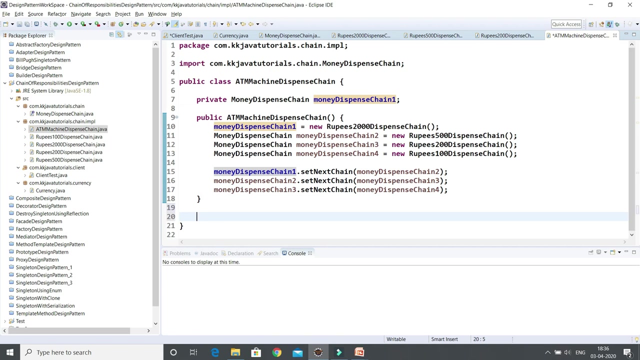 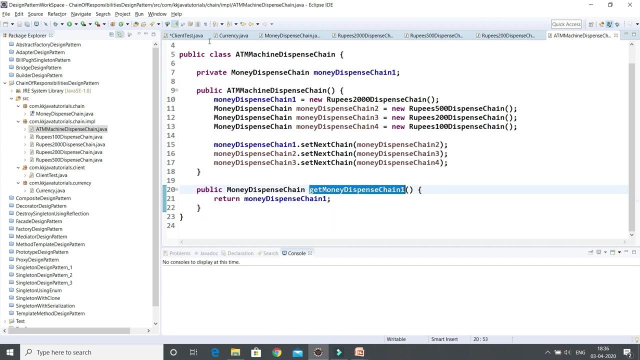 You can call its gator method. Why this is not accessible, Okay, okay, we have provided gator method on the wrong place, I think, I think. I think Here I have provided, so I was supposed to provide gator method here. Okay, so Now we can access this gator method over there. 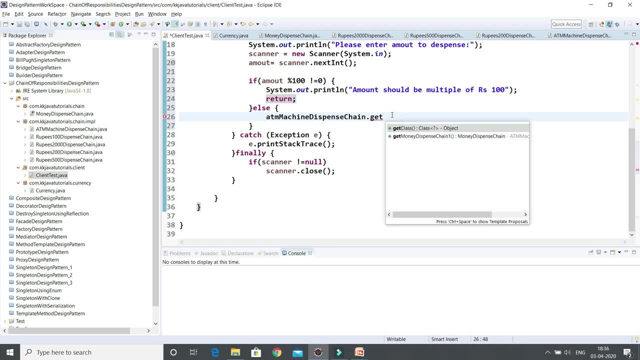 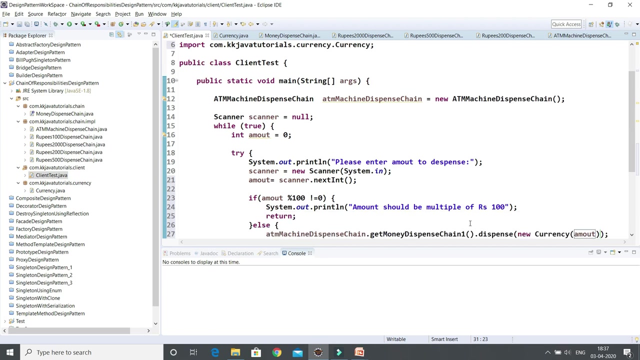 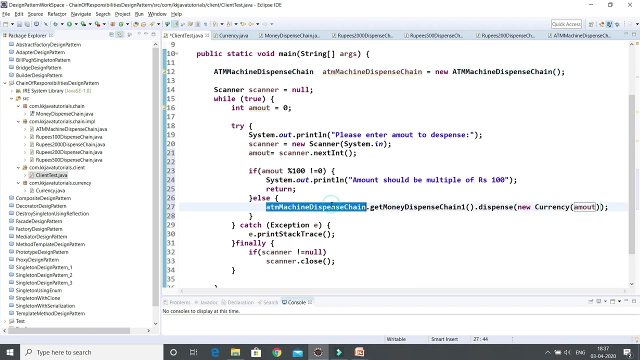 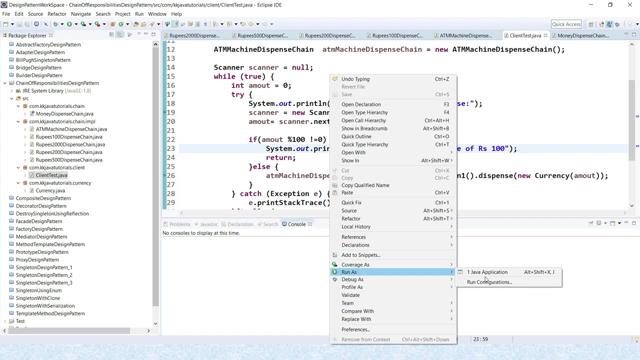 So now we can access this gator method over there. Now we can call dispense method right and Dispense method. there we can create a Object of currency and there we can pass this amount. cool Hope. things should be clear. So here, when we run this line program, let's see what's the output. Let's say we are. 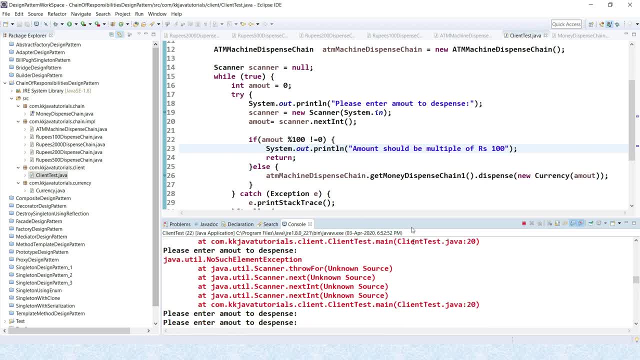 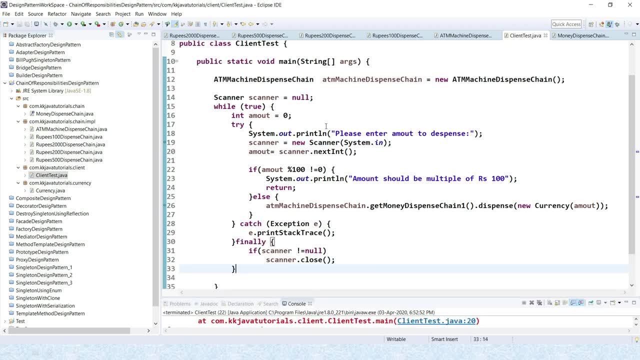 supplying them on 2000, then We are not getting any expected output. reason is that here, if you look into the client program, here come out we have initialize with zero inside the Log. we are just applying the amount as 2000, right? so this condition will be false and 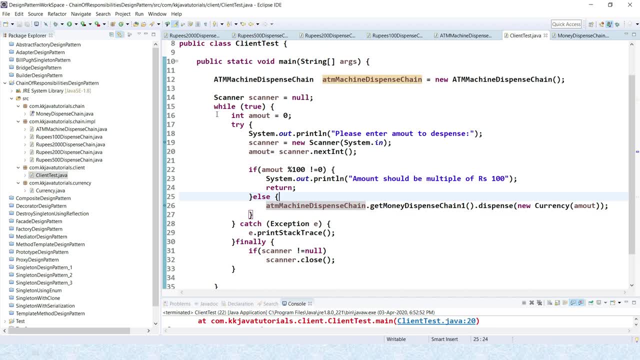 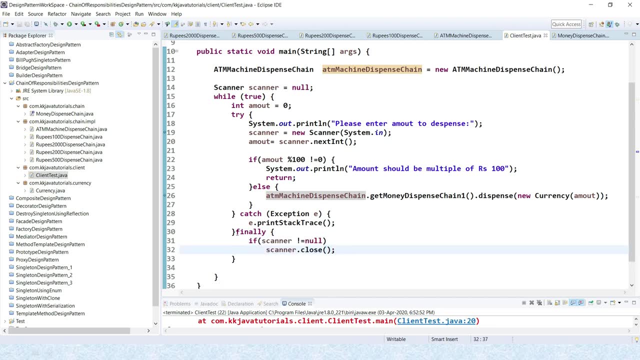 This and that control will go to the house part and after processing, Again control will come and that will try to close these resources. That's the reason This closing resources we can avoid, right. so closing resources is the problem that is trying to close the resource and 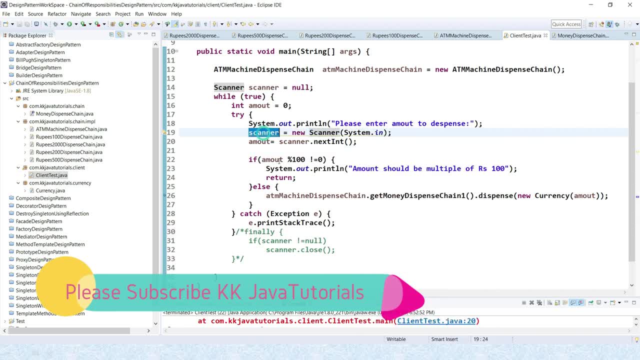 This problem is coming. This problem is coming, so this closing resources. we can close the resource base of the certain condition we can ask. this problem is coming, so this closing lorcrs: we can close the resource Fraser, ah, certain condition. we can ask User, if you want it, Would you like to exceed the? 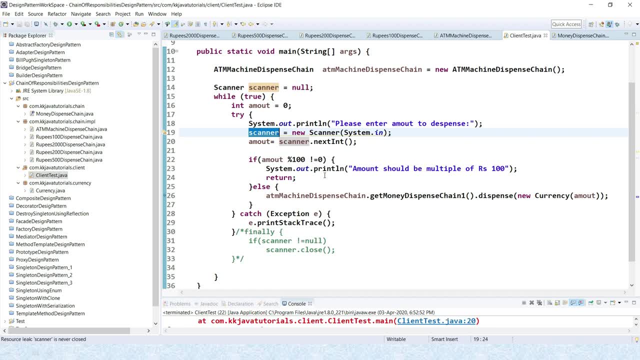 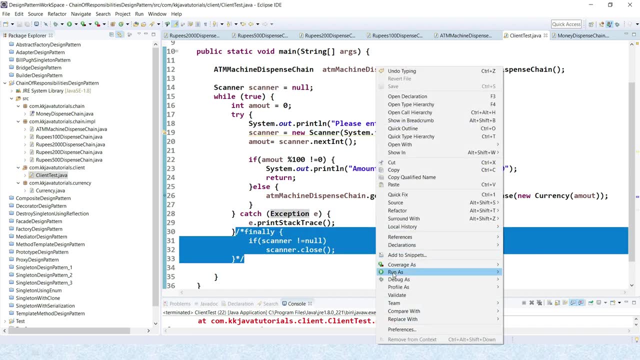 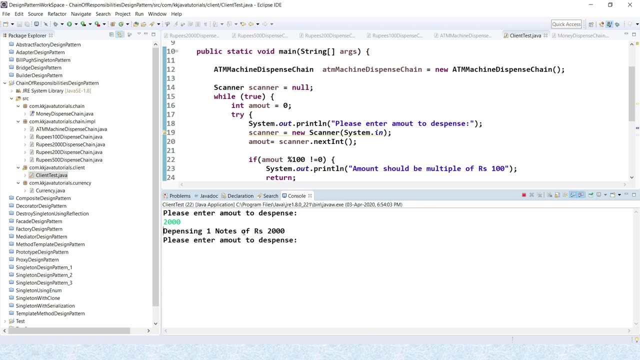 Process. then user may enter some number, hope, and based on that number we can call, we can close this resource. Right now just I'm commenting this closing resources and after that if I run this application Write and let's say user is trying to withdraw 2000 rupees, then here you can see dispensing one note, one note of rupees 2000. right, let's say i'm 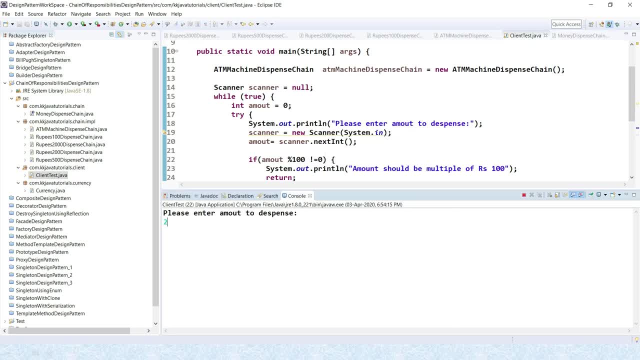 going to uh dispense amount, let's say 23, 000, right? so here you can see: one note is withdrawn for 2000, then uh, one note for 200 and then remaining one note for 100. here you can see how it's uh processing the request. all right, let's say i'm trying to do 12, 12, 30, so this is not possible at. 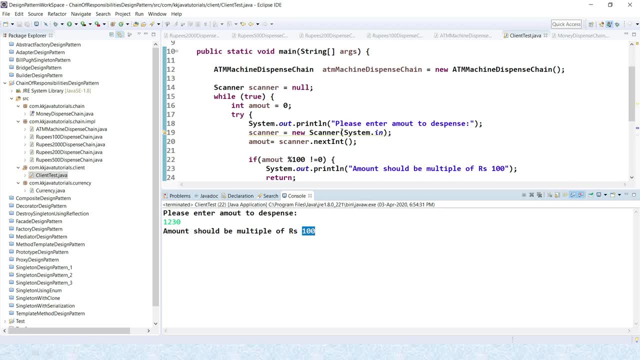 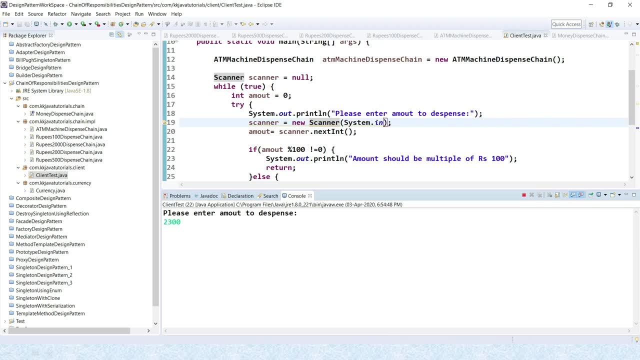 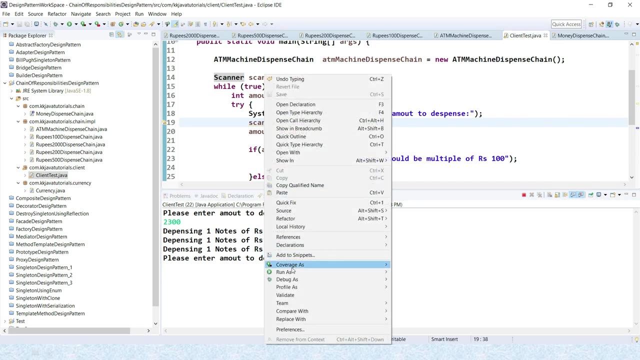 all. so amount should be multiple of uh 100. that is getting printed right. let's say i am again entering. let's say amount, let's say 2300. that's possible to withdraw right. so here you can say one note for 2000 and one not for one, 200 and uh remaining note for 100. now i'm going to process little. 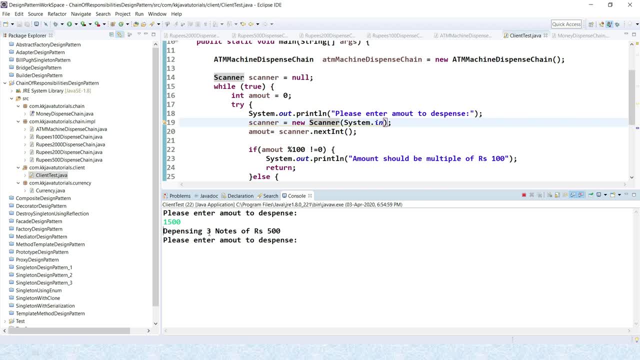 bigger amount. there's a 15 000.. so here you can say: three notes for- uh, here there is some problem, right? okay, fifteen hundred. okay, we don't fifteen hundred, so that's fine. three notes for five hundred. now let's say fifteen thousand, not fifteen hundred. i'm going to enter fifteen thousand, so now this will work for all. 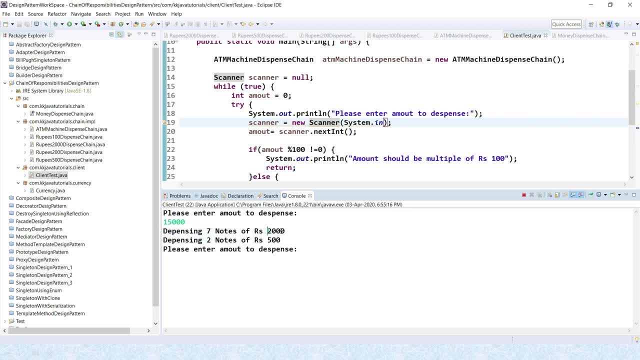 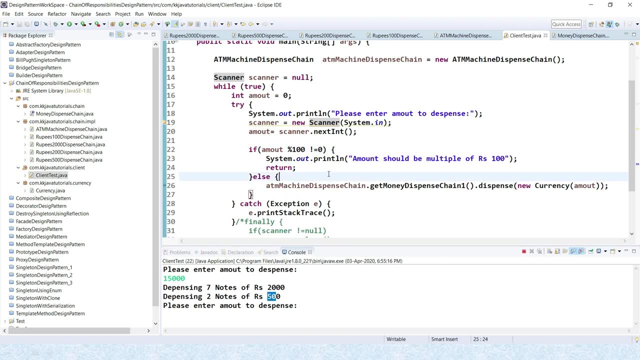 kind of requests. so here, seven notes for two thousand means fourteen thousand, right, and two notes for five hundred. so this code is going to work for any kind of amount, right? which is multiple of 200, which is multiple of 100, right? so, guys, there are a lot of source. 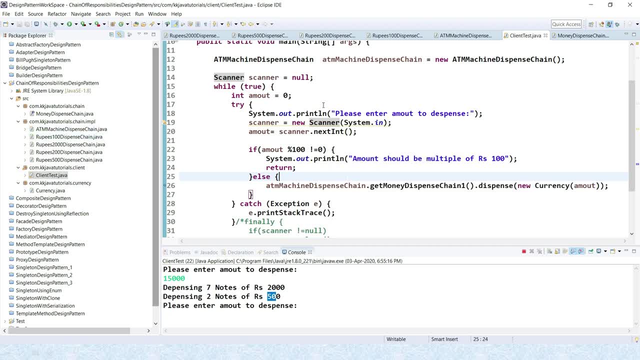 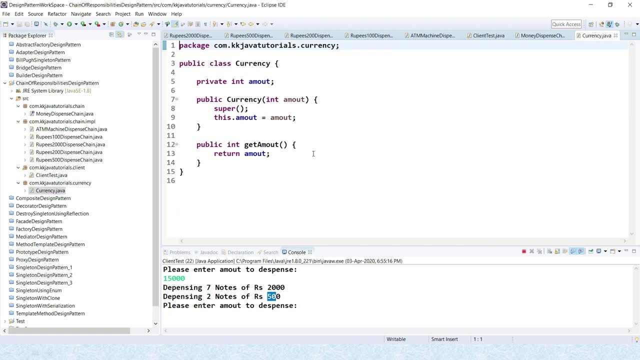 code. i have read it from scratch. uh, here i'm not going to explain each and everything again. i hope you understood. so this is pretty simple. first of all, i have created one currency class which represents amount which is going to use by the money dispense chain right and which is 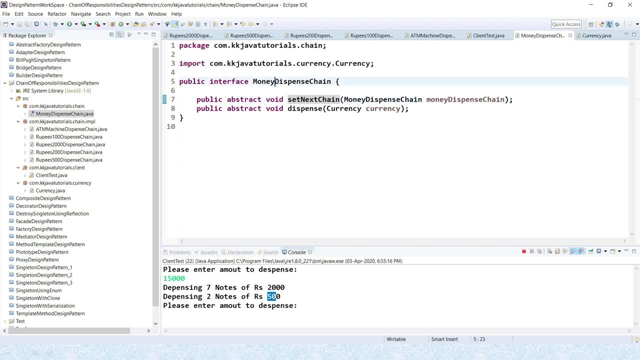 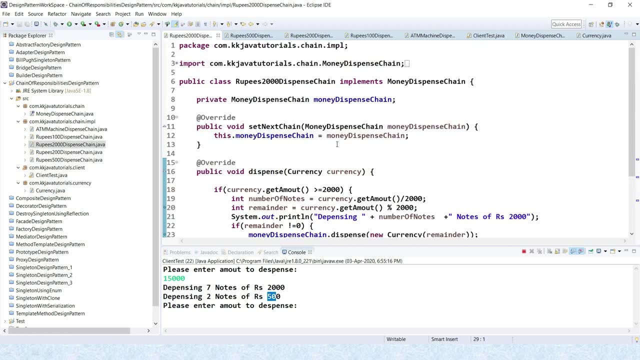 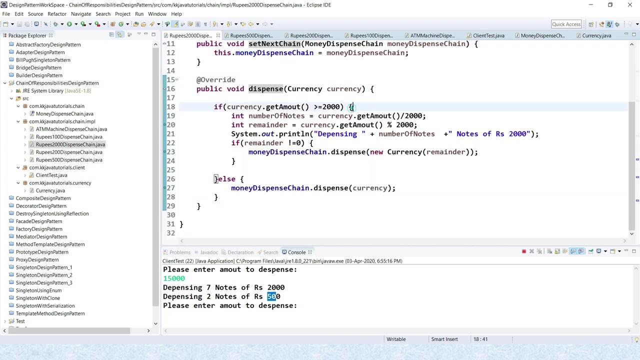 having two methods set: next, chain, which is a reference of money, this machine itself, and dispense having reference of currency. initially i have implemented uh one processor class which is going to process two thousand node and that implements this guy, uh, money dispense chain. and here we have to override these two methods. so main is this one. so if amount is greater than 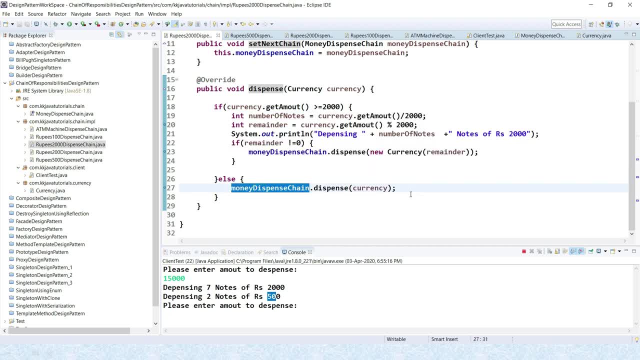 two thousand, then we are going to do this kind of process, else we are going to forward request to the next processor in the chain. right and sorry, uh, if, um, If amount is greater than 2000, then first of all, number of nodes we are getting and 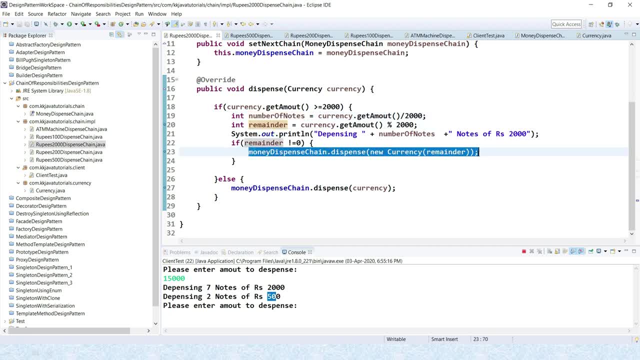 then remainder, we are getting for remainder, we will call the next processor in the chain. If that is not the case, if amount is less than 2000, then we are. then this process is not going to handle, right? If amount is less than 2000, then just we are calling next processor in the chain and passing. 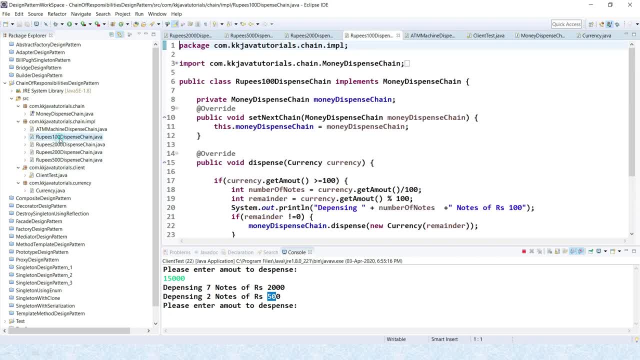 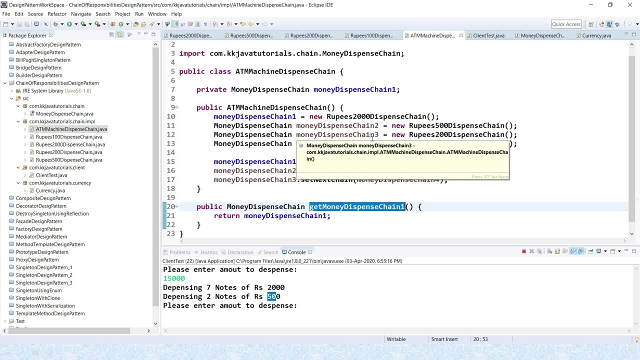 the currency. In similar fashion I have created the rest of the processor classes and finally I had created ATM machine dispense chain there. This is very important. So how you are going to make the chain So here, chain 1 represents the which is processing for 200 node, then as 2000 node, then process. 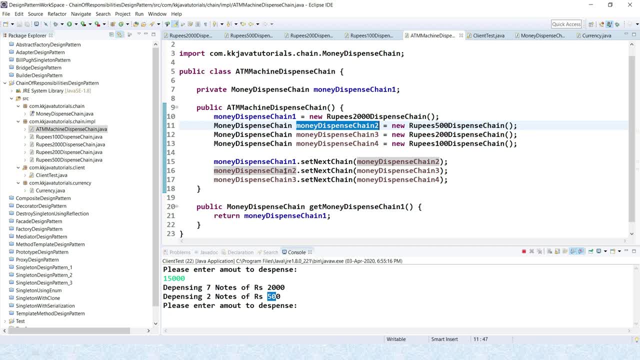 chain 2 is going to process 500 node and similar that And here chain 1 is basically making basically that. that is, that is a point that is basically setting chain to the to the Chain 2, and then chain 2 is setting reference to the chain 3 and chain 3 is referencing. 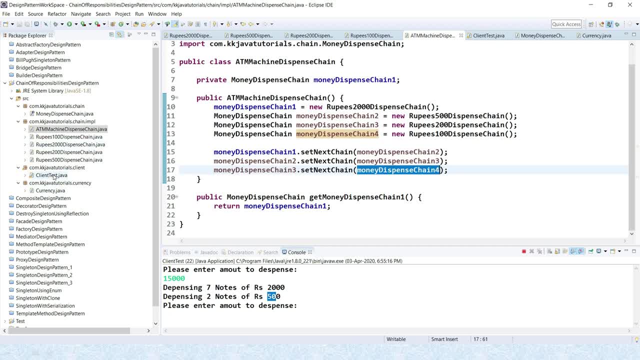 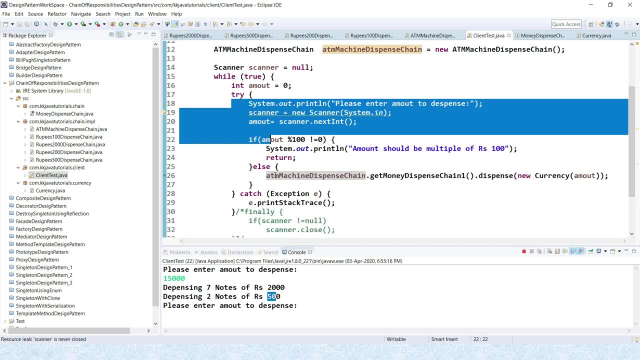 setting reference to the chain 4, something like that, right. And finally we had a client program and there I have created an instance of ATM machine dispense chain. there, just I am taking the amount right. If amount is not multiple of 100, just I am printing this message and exit the process. 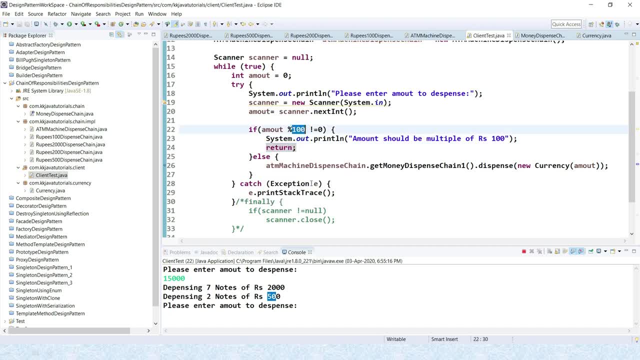 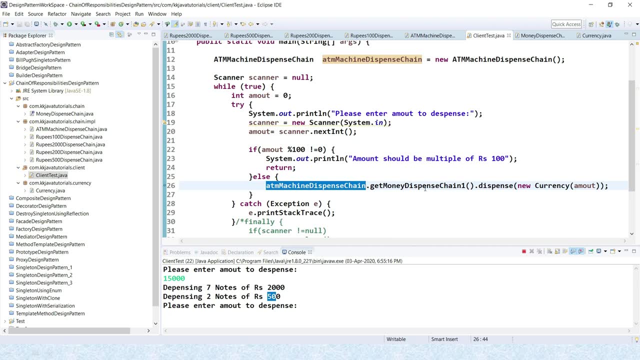 If amount is basically multiple of 100, then we call, We write this, We write this, We make use of this, basically class. there we have a reference of first chain right, This is the first chain in the chain, So we get the reference of that and we are calling the dispense method by passing the. 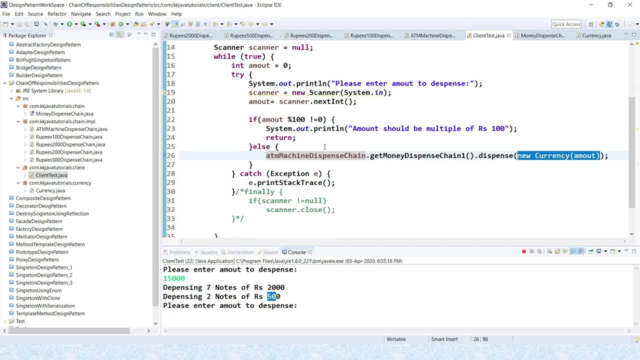 currency amount right And that's the way basically entire chain is working. So I hope you understood. If you have any question or any doubt, then then you can post your queries below to the video. I will try to answer you. As far as source code concern, I will post this source code on my blog, kkjavacom. and. 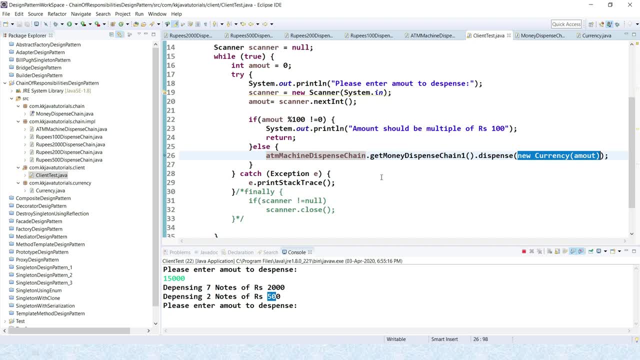 you can download from there. Guys, big thanks for watching this video and see you there in the next video tutorial. 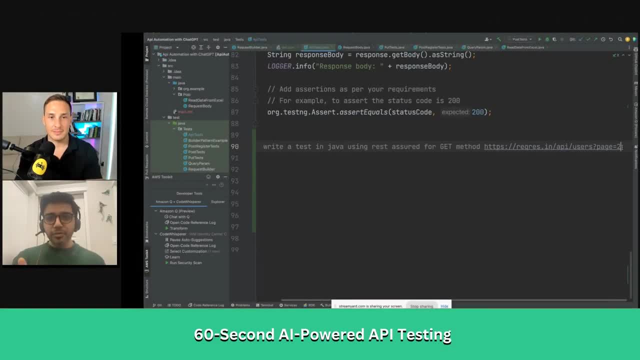 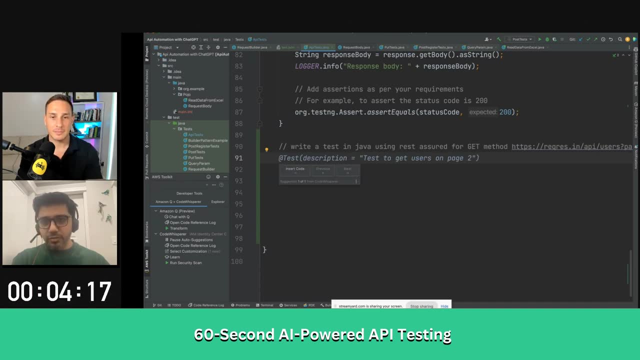 Let's give it a try- that how we can write a automation script using rest assured in Java for get method And for demo purposes. I am using this endpoint. Okay, this is an open source endpoint. you folks can also use it, there is no harm in it. So this is the prompt I have given, that write a test in Java using rest assured for get method, right? So, if you have noticed, it has already prompted me at the test description. So see, AI is pretty smart, right? It is using description, which we folks miss a lot. Okay, so I have. 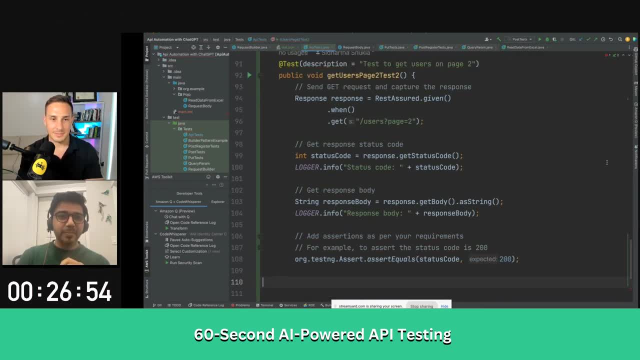 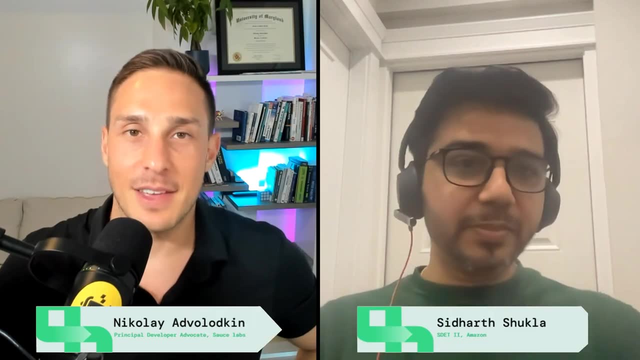 and press enter again And after you press enter, see, So I guess it doesn't take even 60 seconds. it has completed writing the code in just two or three seconds. Sid, do you think you can code- and a rest assured- API test- in 60 seconds?